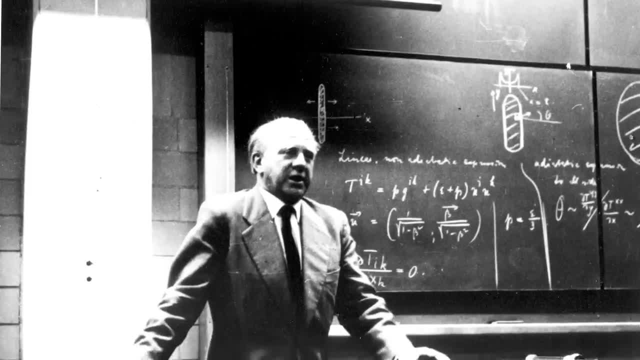 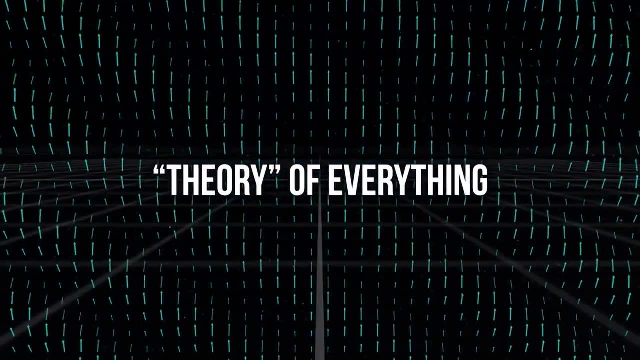 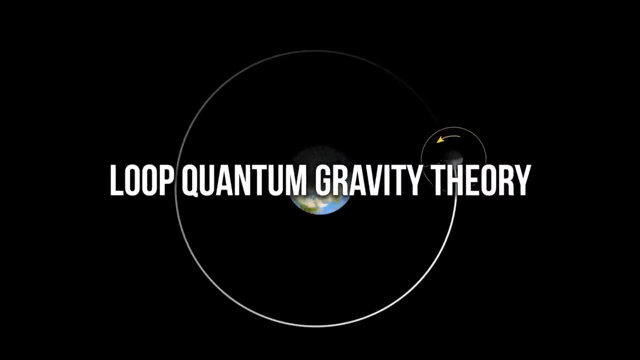 thought experiment about the superposition of quantum states and Heisenberg's uncertainty principle. But the holy grail of scientific research, a so-called theory of everything, has repeatedly crashed against the apparent impossibility of a quantum gravity theory. Of course we have loop quantum gravity theory aiming to reconcile quantum mechanics and 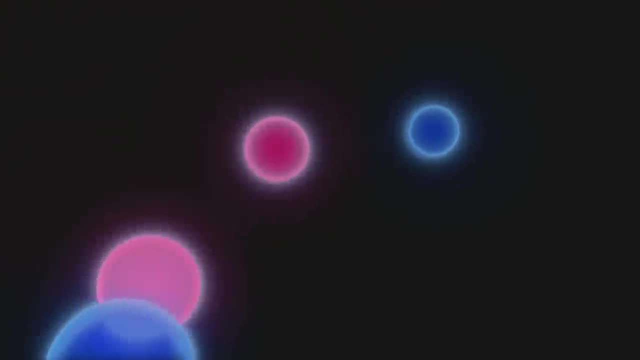 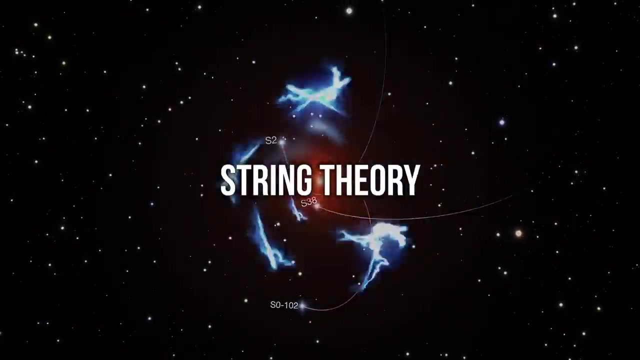 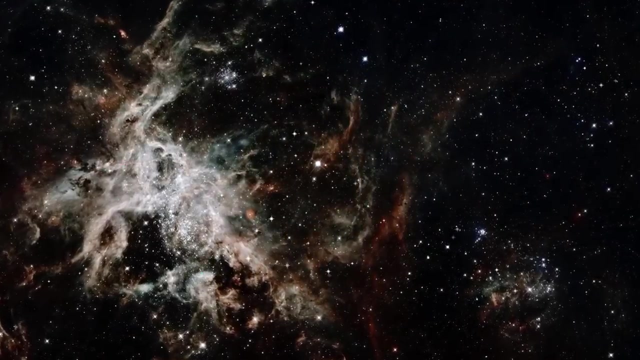 general relativity, but a definitive quantum-based explanation of spacetime is yet to come. But let's rewind a little bit to understand how quantum physics evolved into string theory as it tried to integrate the complexities beyond subatomic particles and their connection with the now-old classical mechanics. Is string theory the road to the ultimate standard model? 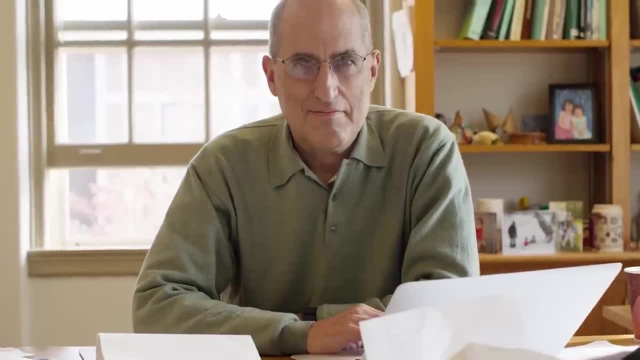 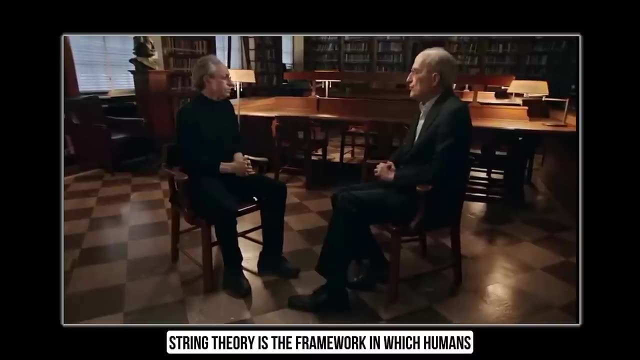 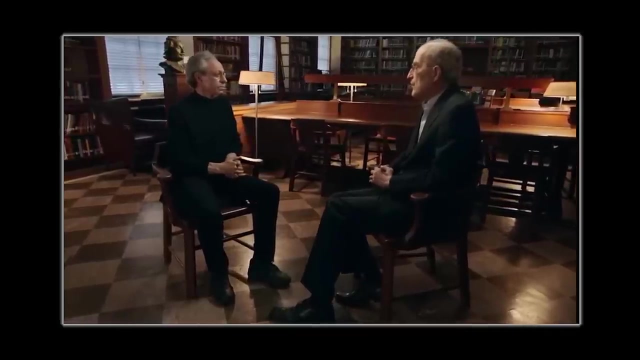 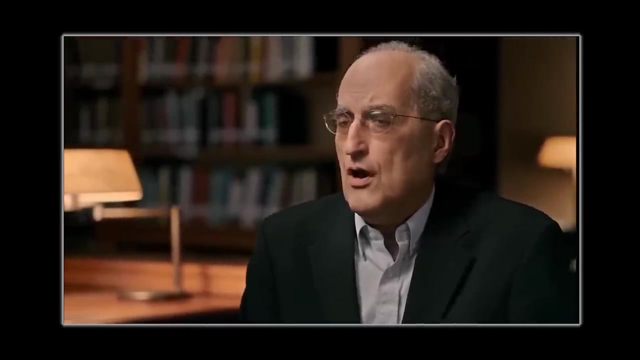 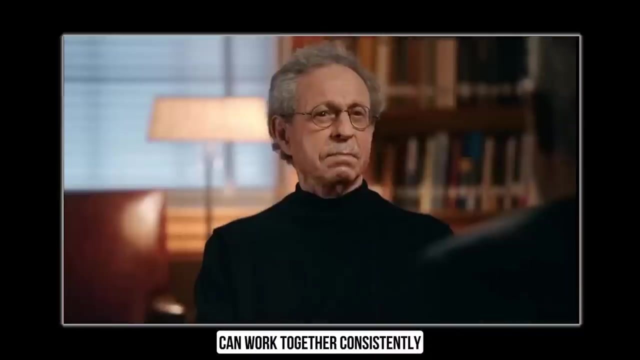 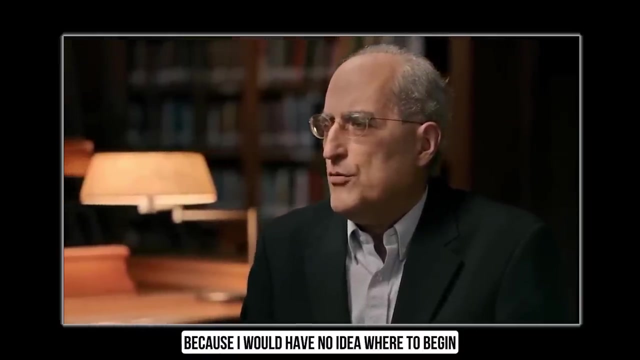 or do we need a new paradigm shift? American physicist and mathematician Edward Witten has a lot to say about the gravity of the situation. If string theory had not been discovered, I personally think that I would not have tried to discover something like it, because I would have had no idea where to begin in reconciling. 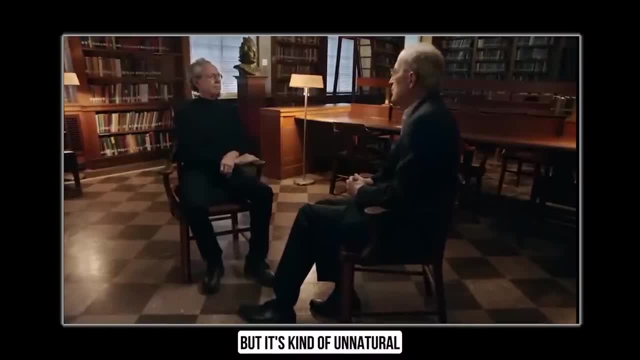 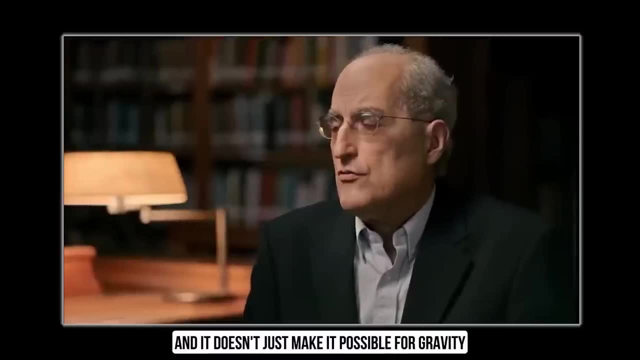 quantum mechanics and gravity. But it's kind of unnatural to ignore the fact that there's an extremely rich theory that people actually have discovered that can make this work. And it doesn't just make it possible for gravity and quantum mechanics to work together, but it 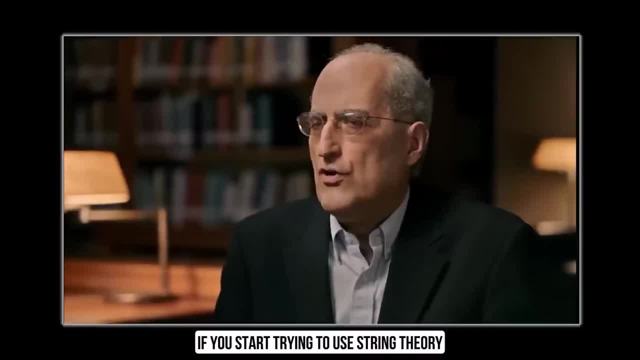 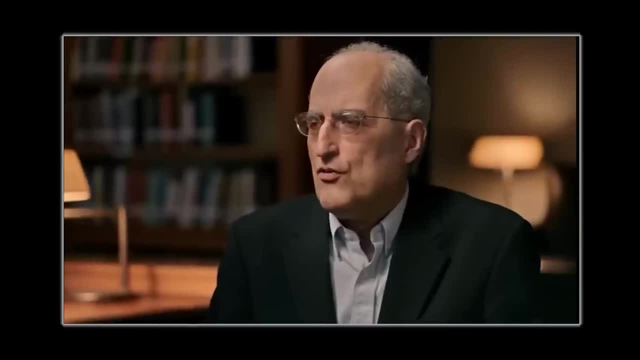 forces them upon you If you start trying to use string theory to describe a quantum theory that you think maybe doesn't have gravity. gravity is literally forced upon you because of the way it pops out of the equations Quantum Field Theory vs String Theory. 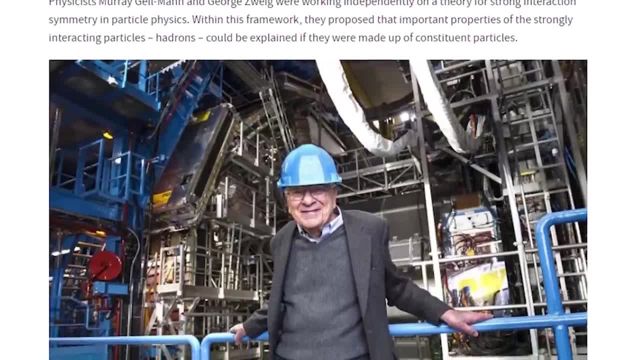 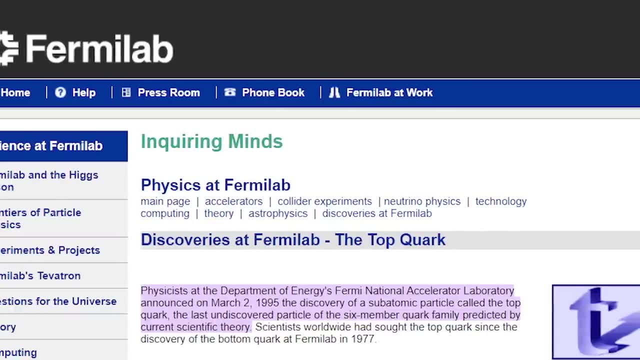 When protons and neutrons were dethroned as elementary particles, both theoretically by Gelman and Zweig's proposals in 1964 and Fermilab's last quarks discovery in 1995, a seemingly infinite array of possibilities emerged from the mysteries popping in and 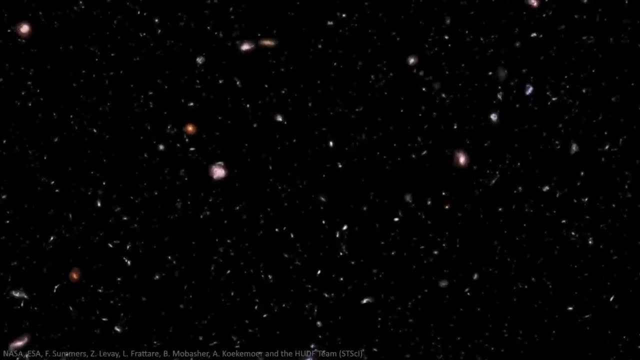 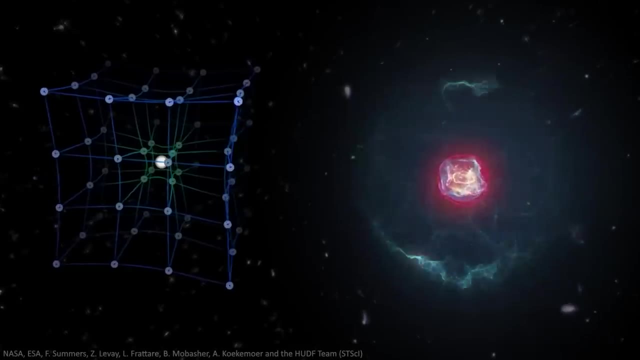 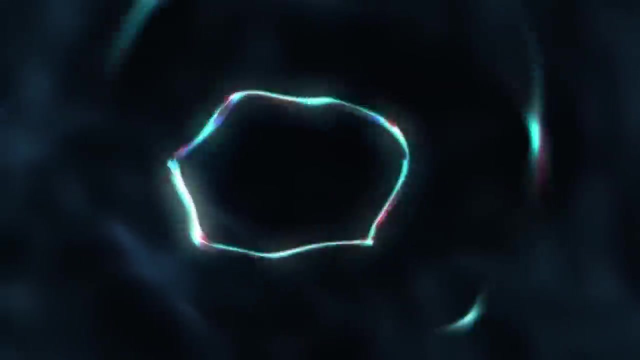 out of existence. at the very Planck's length, It was eventually realized that a new approach called string theory was a promising candidate for a quantum theory of gravity. This theory presented point-like particles in a revolutionary way. They were all but little loops of vibrating one-dimensional strings, Just like a musical. 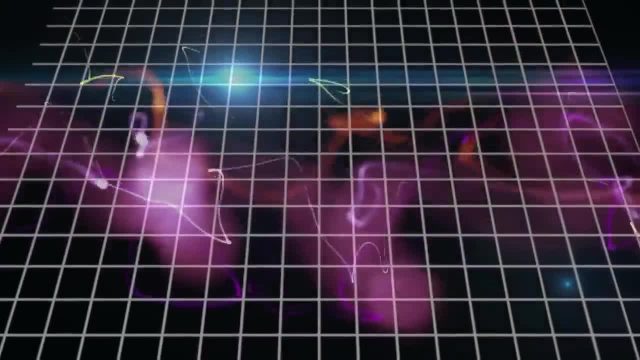 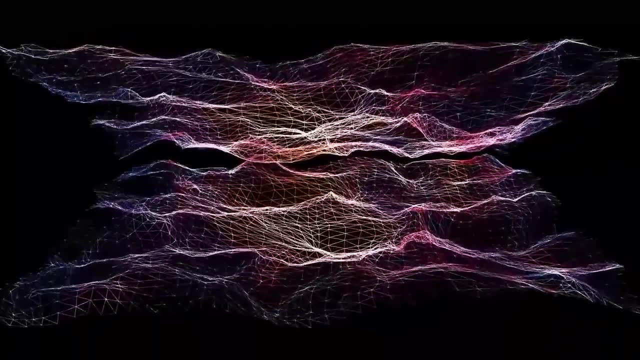 instrument can create different notes using the same string. these one-dimensional objects can vibrate in different ways, thus giving birth to several types of particles. To continue with the analogy, if the different harmonics of the string theory were to be the same, they would be the same If the different harmonics of the string theory were to be. 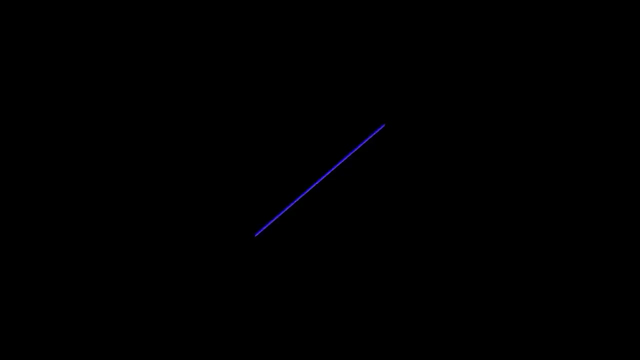 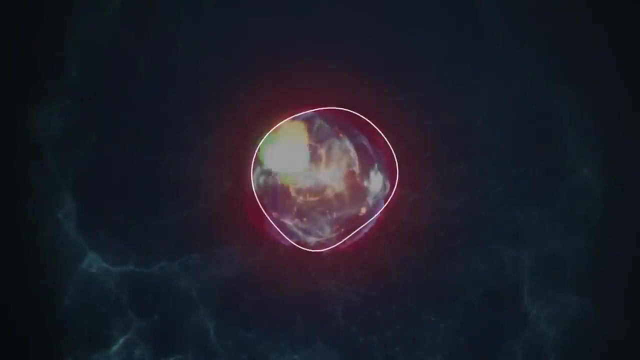 the same, they would be the same. If the different harmonics of different strings resonating at once create the beauty of a musical piece, then the several vibrations of these strings create the building blocks for the neutrons and protons hadrons seen before as simple and elementary. 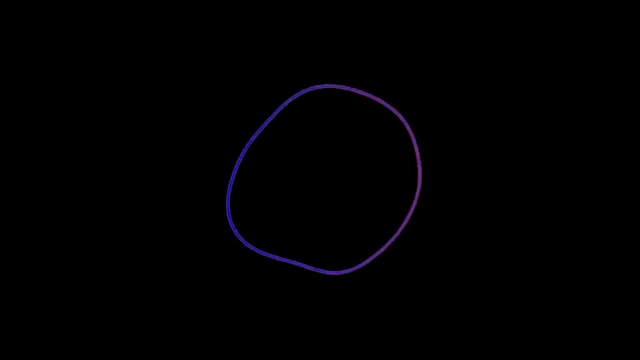 point particles. Now that we have a vibrating string resonating in different harmonics, we identify each of these vibrations as an electron, a photon, a graviton, a neutrino, a specific variant of quark, etc. This creates an elegant approach in 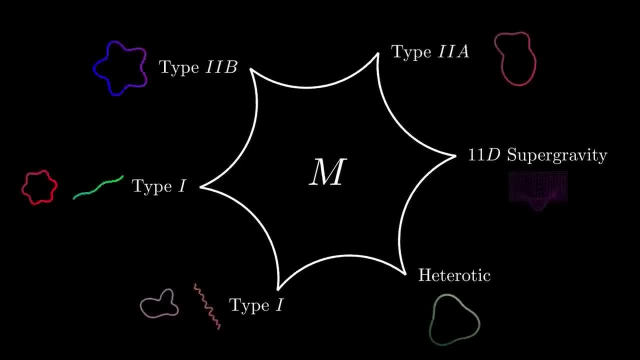 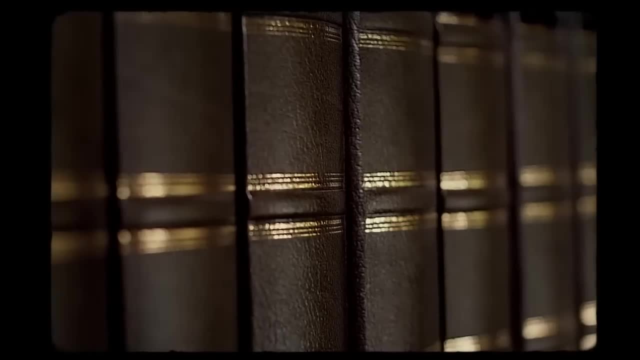 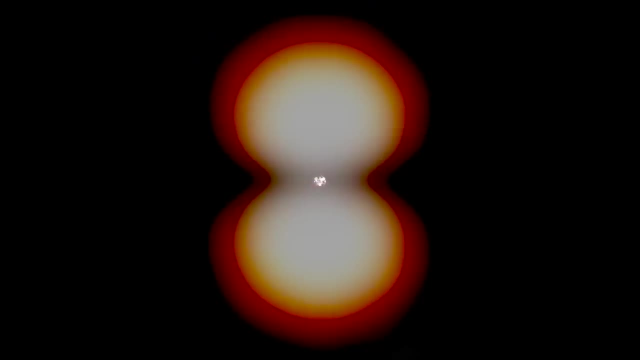 which all particles are created from one basic and ultimate origin. This time there's now going beyond the string. There's no lower level to examine and no further division is possible Using another simplifying analogy, even when there's not a measurable size for a string. 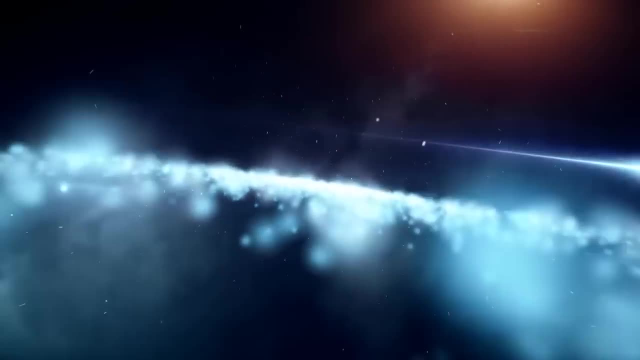 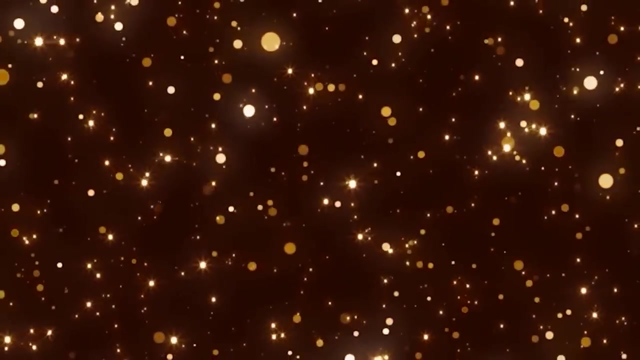 we could say that the scale difference between a string and an atom would be comparable to that between an atom and our entire solar system. But how could such a theory be useful when it comes to gravity? Well, we could say that gravity can be used to measure gravity. 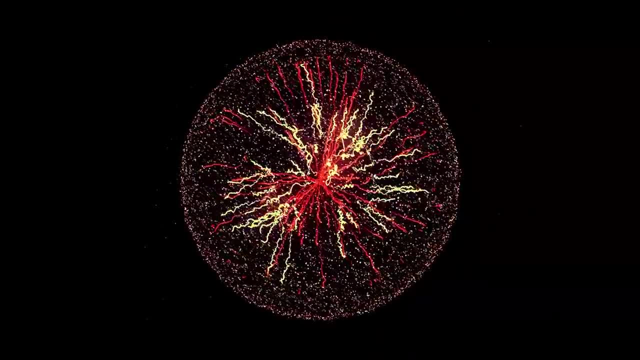 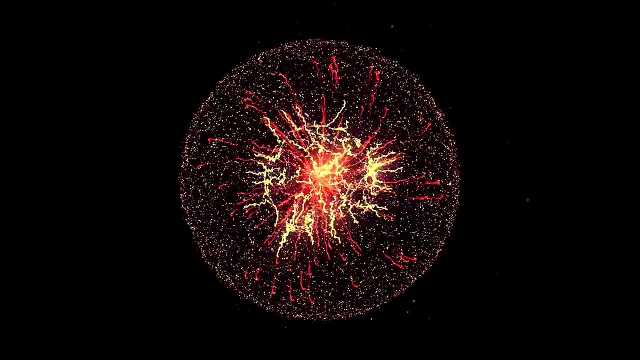 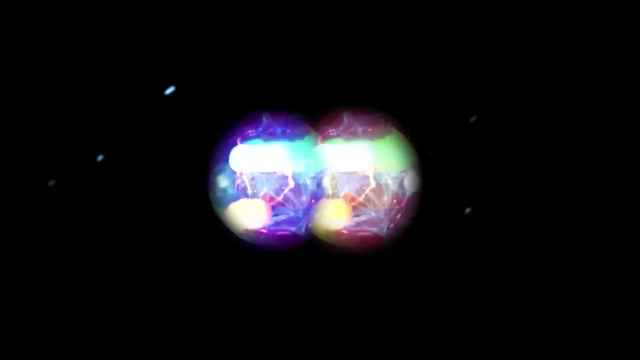 Well, as we said before, one of the vibrational states of the string creates the graviton. If the graviton is a quantum mechanical particle that carries gravity, then string theory becomes a way toward a quantum gravity theory, Just like the fuzziness present in the orbits of classical point-like particles led to further 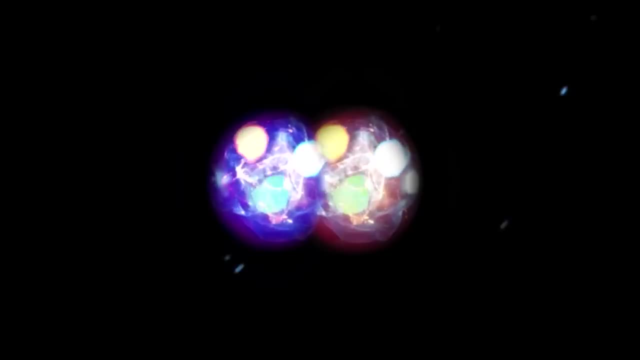 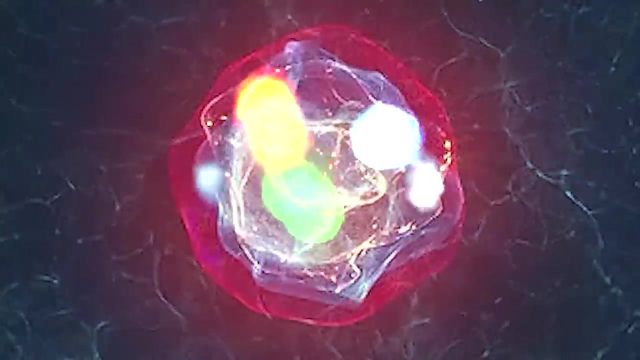 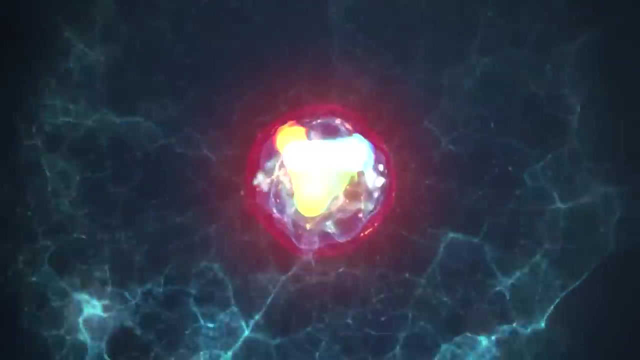 observation and ultimately the realization of a quantum mechanics-related behavior of electrons, which allowed the emergence of solid theories regarding electricity. atoms and molecules can introduce a new type of fuzziness. First, they're interacting like vibrating strings instead of points, And second, they behave quantum mechanically. 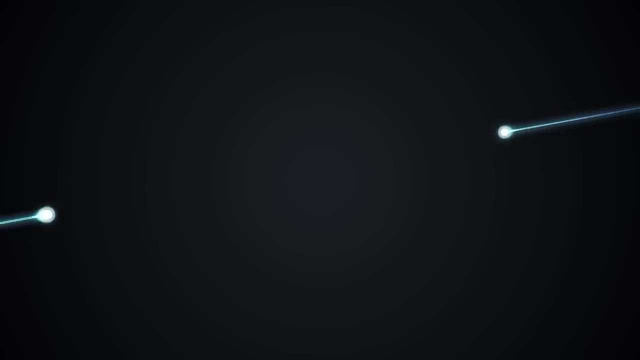 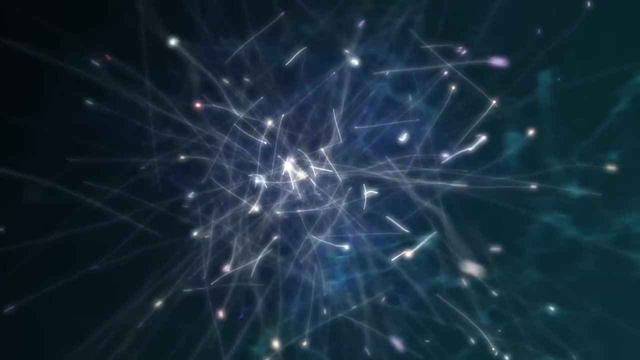 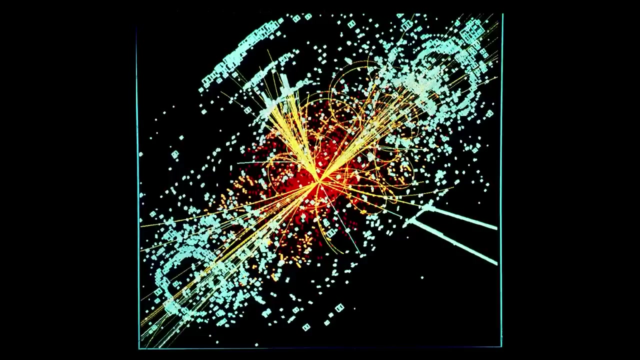 At some point in his career, physicist Edward Witten, regarded by many physicists as Einstein's true successor, thought this to be the key to elaborating deeper into a quantum gravity theory. Gravity would be an inevitable consequence of the string model itself. You see, when you look at particles as classical point-like particles, 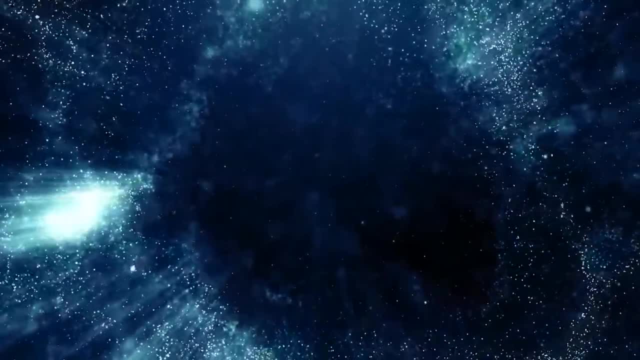 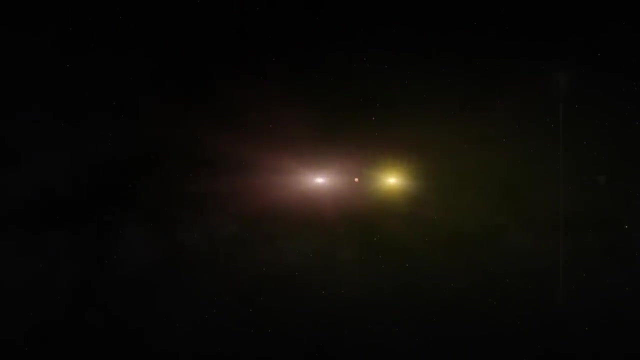 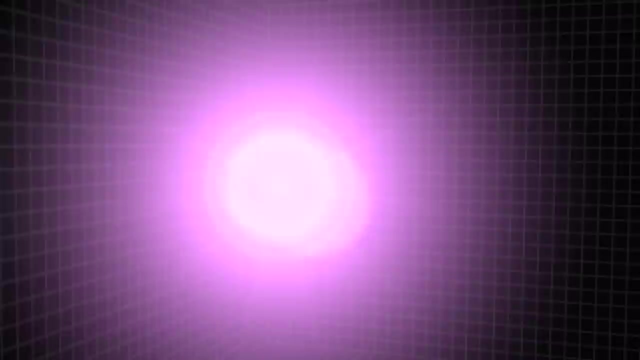 Two particles can join to become something else, or can split to become two different things, But each of these changes is represented by a discrete event at which breaking or joining happens. Knowing what each particle is never tells you how it's going to interact with another one. 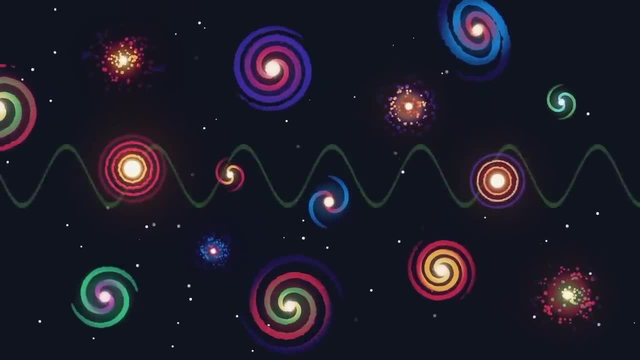 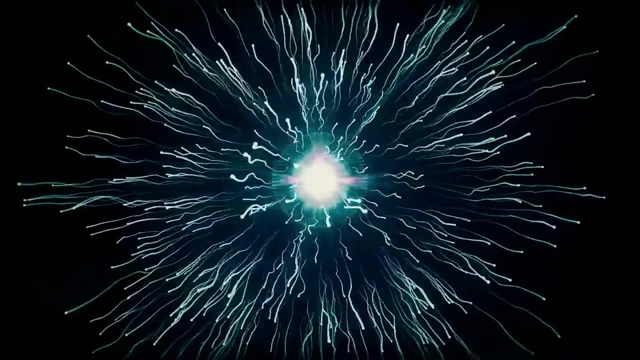 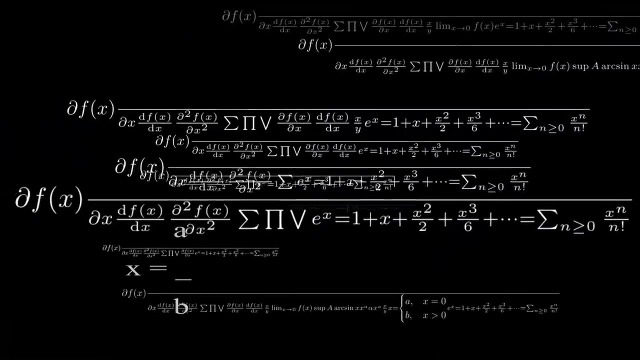 But when you look at particles as strings, there is no scattering, since a string transitions smoothly to a new state in which it becomes two different strings, or vice versa, Drawing a smooth picture of spacetime in which knowing what a string is implies knowing how it interacts. This difference is what, in Witten's words, 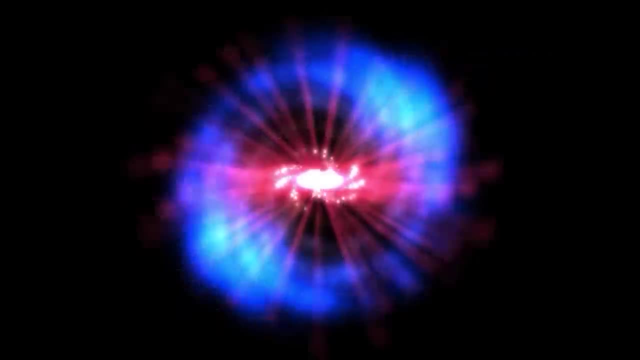 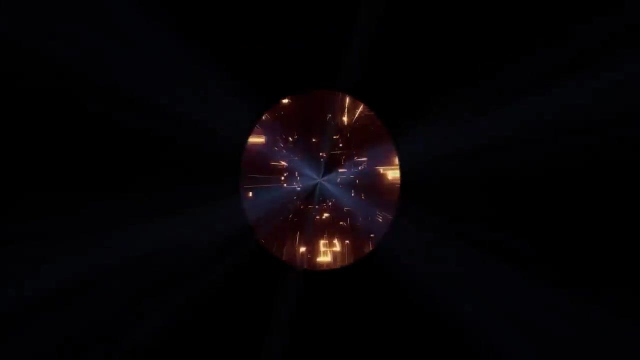 was seen as the germ of the fact that string theory is more predictive than standard quantum field theory. You don't need to separately say what the objects are and how they behave. Once you've said what the objects are, how they behave is completely defined. 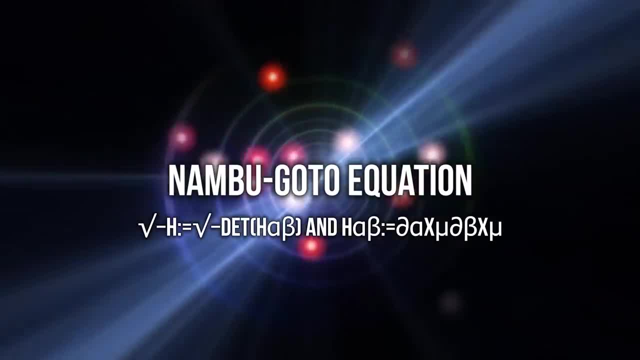 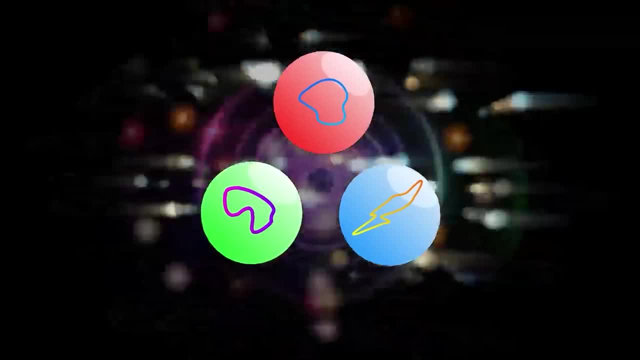 Thanks to this approach, we have the Nambu-Goto equation, which describes that, just as the action for a free-point particle is proportional to its proper time, the length of its worldline, a relativistic string's action is proportional to the area. 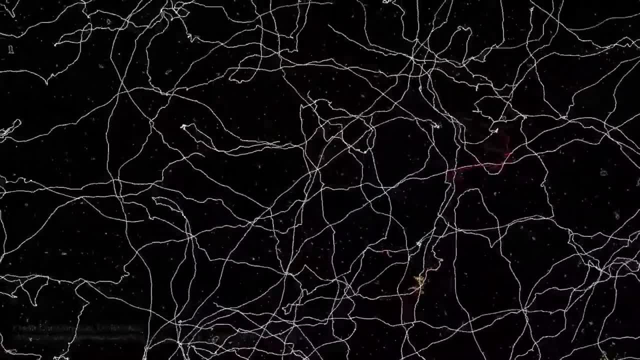 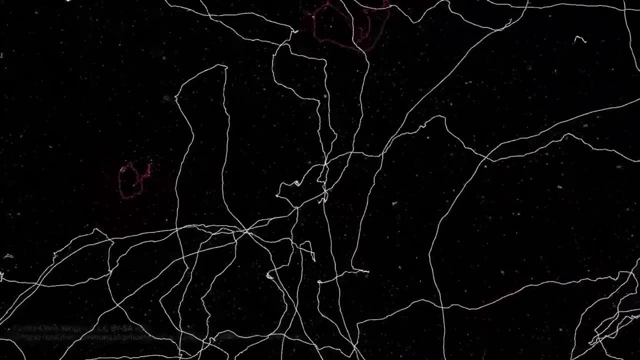 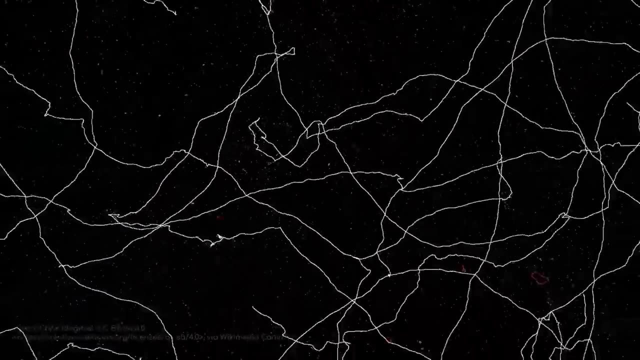 of the sheet which the string traces as it travels through spacetime. Witten used to put this in a somewhat misleading visual analogy. Previous quantum field theory equations describe the movement of something like a rubber band, while Nambu-Goto describes a travelling soap bubble that draws the very fabric of spacetime. 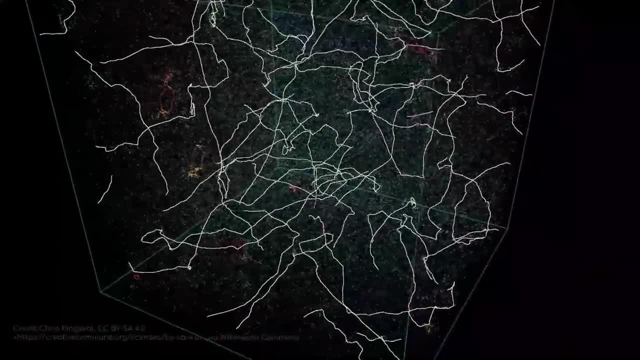 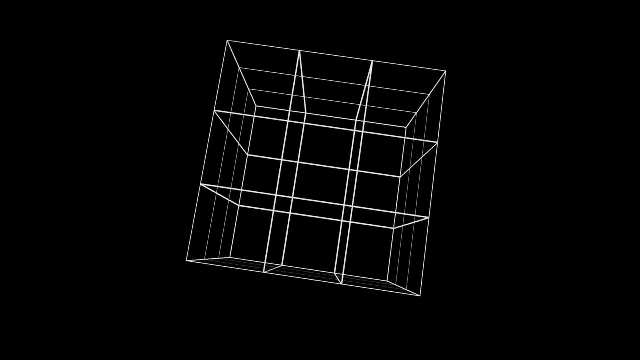 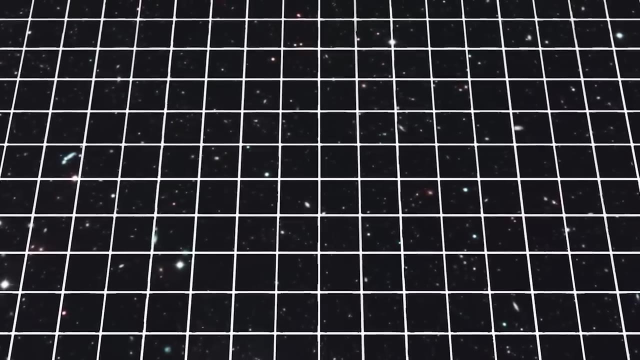 In the first case we only have discrete accounts of what the particles are, but in the second case we have what the strings are and how they behave. But when the problem of left-right symmetry was introduced in the ever-changing fields of string theory variations, it became clear to Witten that the onion still had many layers to peel. 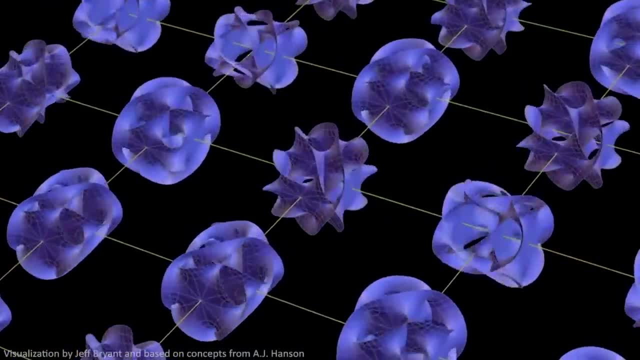 For Witten, the problem has implications so profound that he started envisioning a future where physics would work in terms of something more basic than space and time as we know it. A future is a glue, a naturalallenangillionаниеsomethingmorebasicthanspace andtime as we know it. 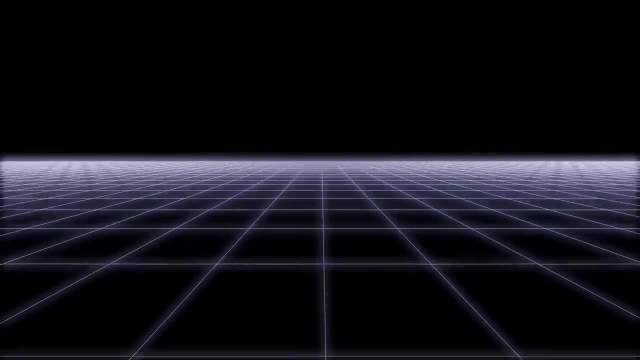 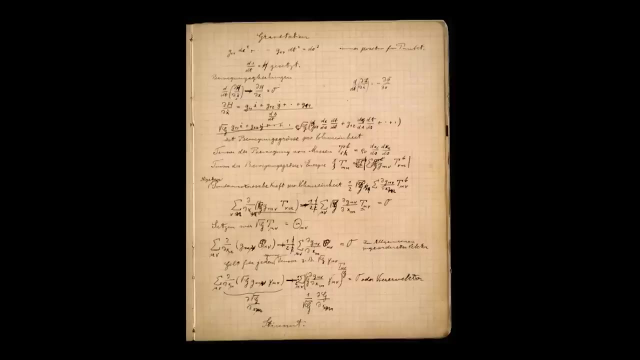 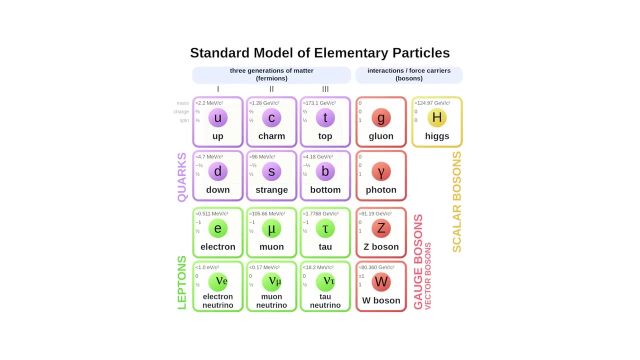 future in which spacetime would become as fuzzed up as position and velocity became with the rise of quantum mechanics. This all signaled for Witton the need to understand at a deeper level what space and time really are, if one wishes to comprehend those regions of reality that remain a question today. such 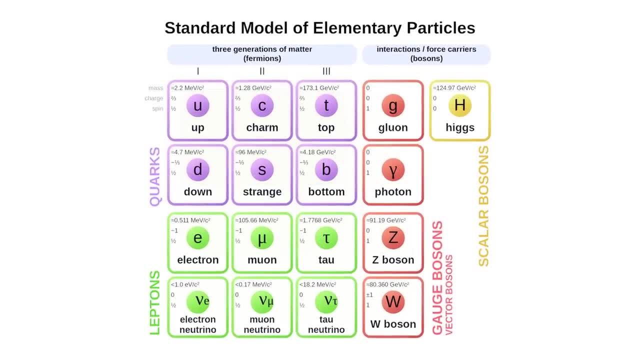 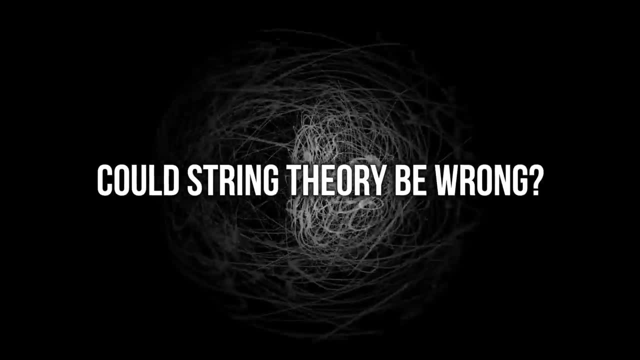 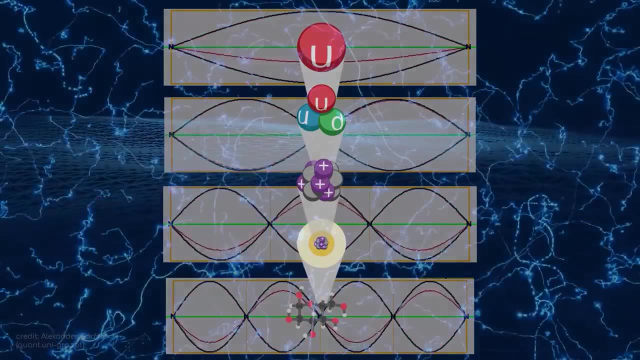 as black holes, the ultimate structure of elementary particles or the moment before the Big Bang, where the concept of time itself breaks apart. Could string theory be wrong? One of the main criticisms of string theory is that it can't be tested. According to Witton, we have the theory's prediction of supersymmetry, an extension. 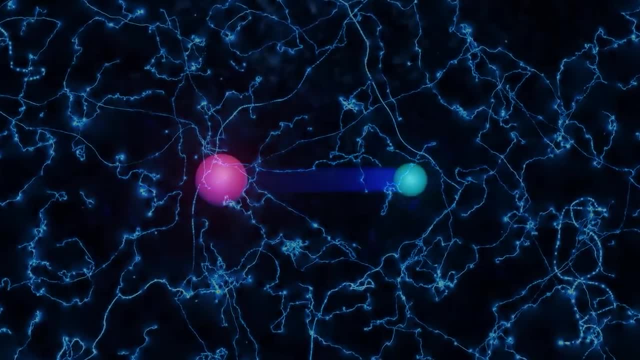 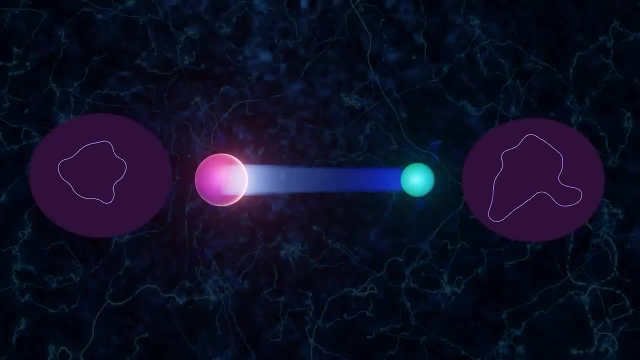 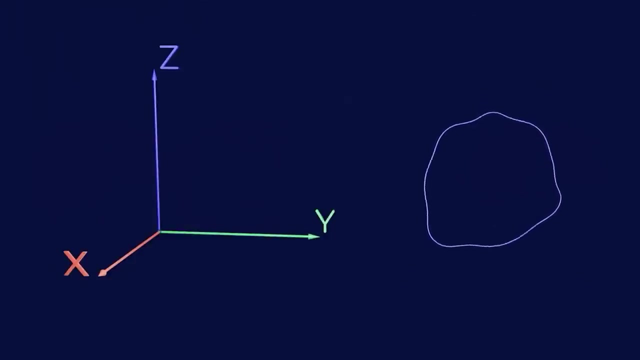 of the standard model that aims to fill some of the gaps by predicting a partner particle for each particle in the standard model or, put differently, a theory in which the equations for force and the equations for matter are identical. Witton hopes that this is the decade when supersymmetry will be discovered, but he kinda. 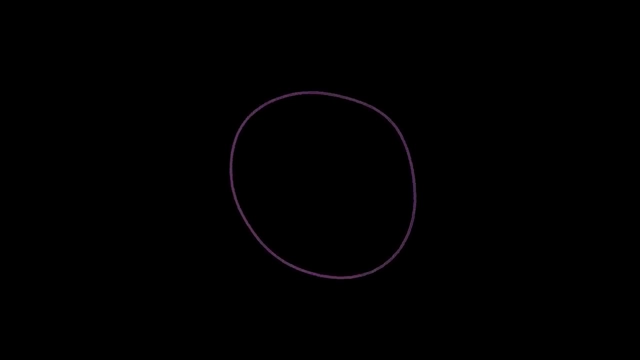 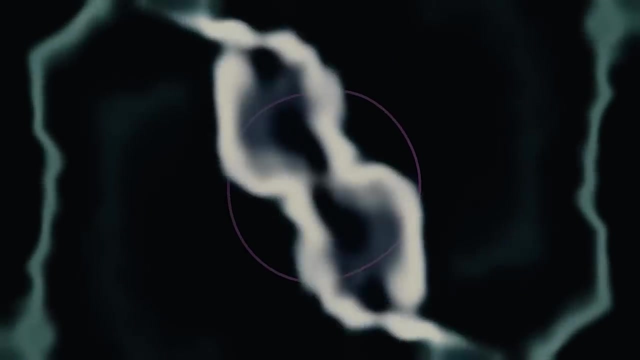 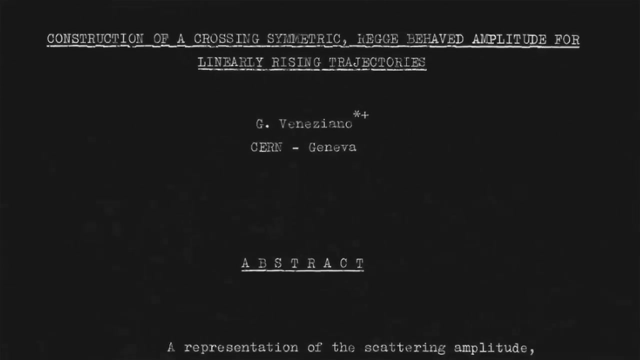 leaves it to speculation. New technologies, New methods And new instruments could surprise us in the years to come. But despite the theoretical appeal of supersymmetry, no experimental confirmation has been obtained so far, And the experiments conducted at the Large Hadron Collider have excluded even the most. 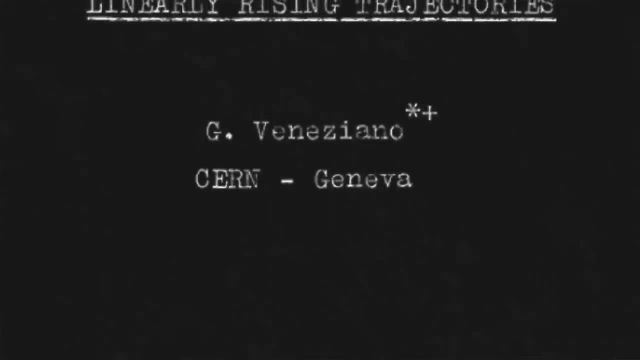 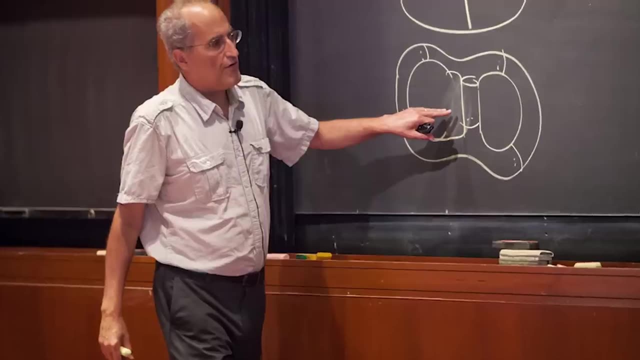 straightforward supersymmetric scenarios. There's still a big possibility for string theory to be wrong, and Witton himself recognizes it in an interview for NOVA. I guess it's possible that string theory could be wrong, But if it is in fact wrong…. 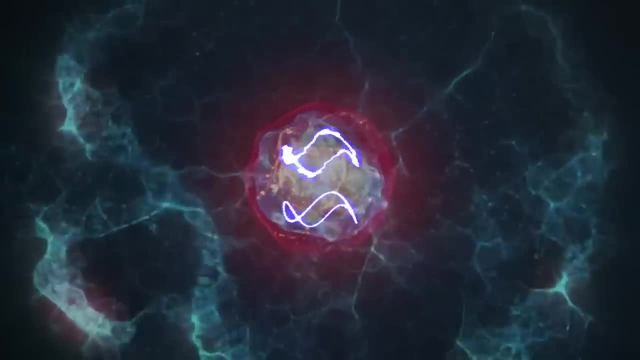 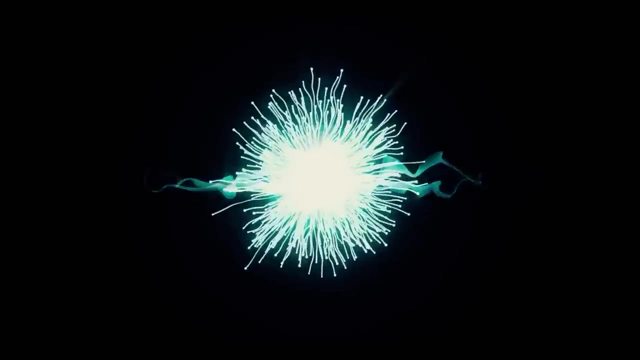 It's amazing that it's been so rich and has survived so many brushes with catastrophe and is linked up with the established physical theories in so many ways, providing so many new insights about them. I wouldn't have thought that a wrong theory should lead us to understand better the ordinary. 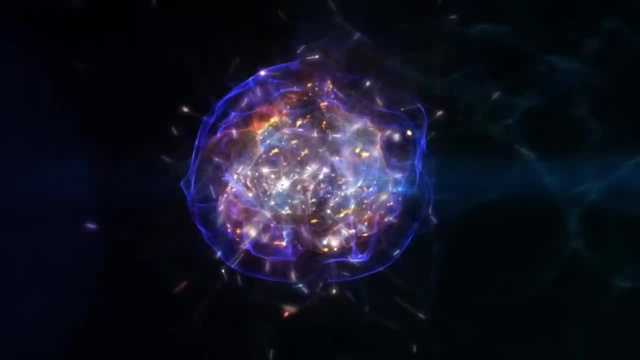 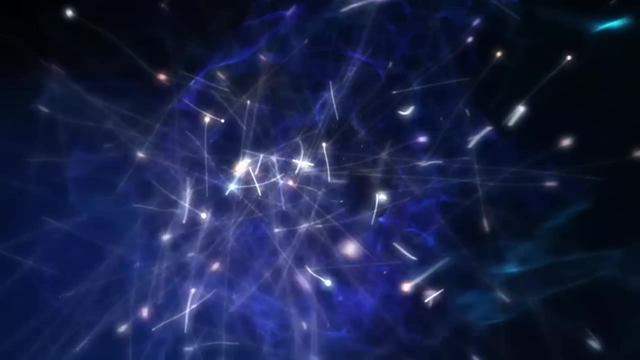 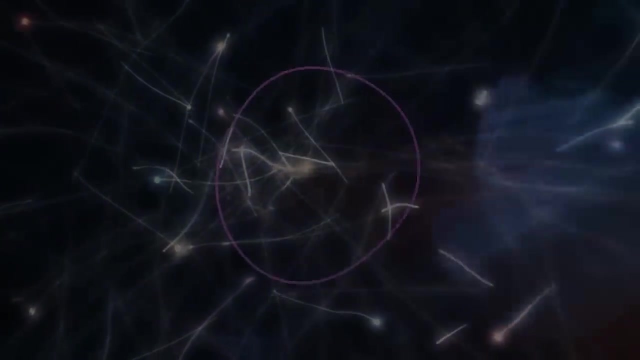 quantum field theories or to have new insights about the quantum states of black holes. Witton's belief in string theory went as far as to compare the odds of the theory being wrong with disproven assumptions made in the past by people claiming that fossils were put on Earth by a god trying to test our faith. 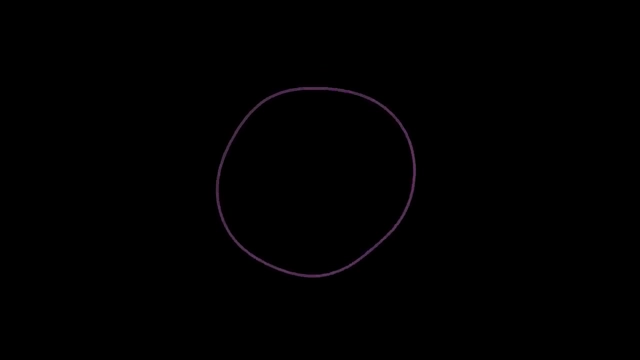 He said string theory might be wrong, but it would seem like a kind of cosmic conspiracy. He seemed hopeful, though, comparing the field to a slow-paced puzzle meant to be patiently solved by people who didn't have a clear idea of the final picture they were aiming. 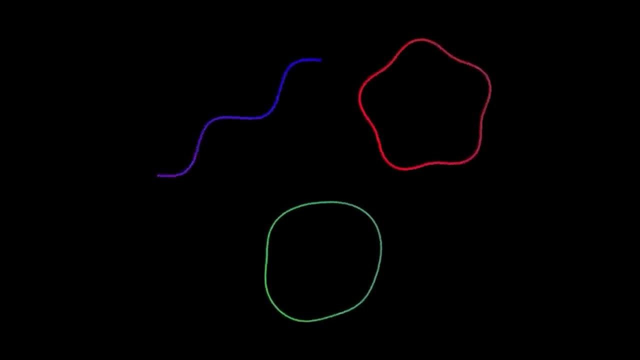 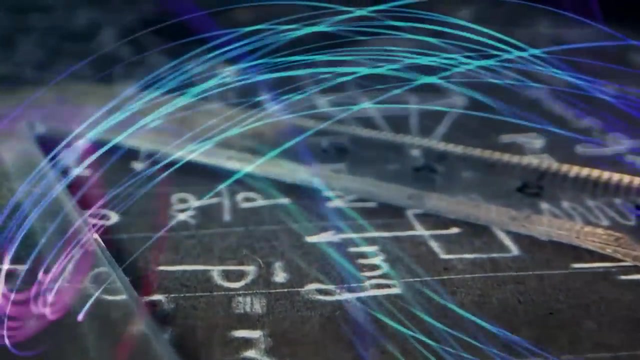 to form when they started. Could this difficulty to prove the theory result in a career shift for someone like Witton, who's dedicated his life to it? It's been noted that in recent years, Witton may have shifted his focus to condensed matter. 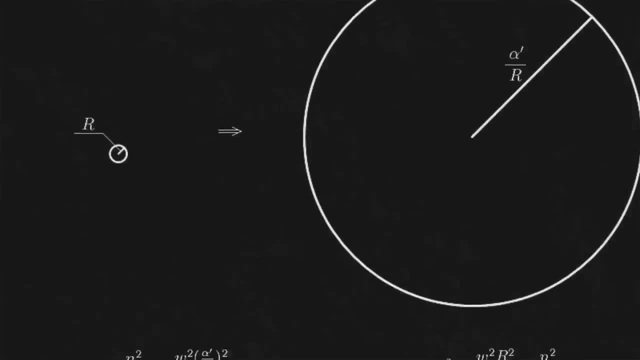 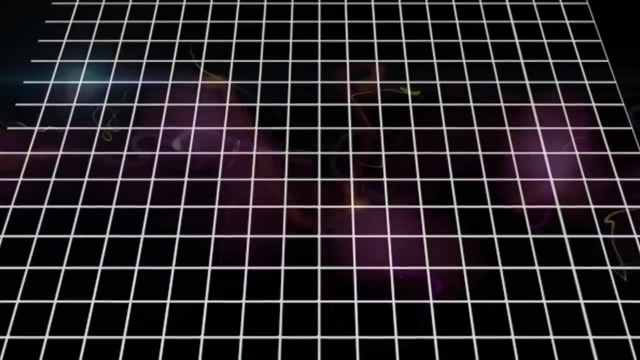 physics Witton has described his interest in this field not as a complete career shift, but instead as a natural extension of his work in string theory, as many concepts and techniques used in string theory can also be applied to the study of condensed matter systems. 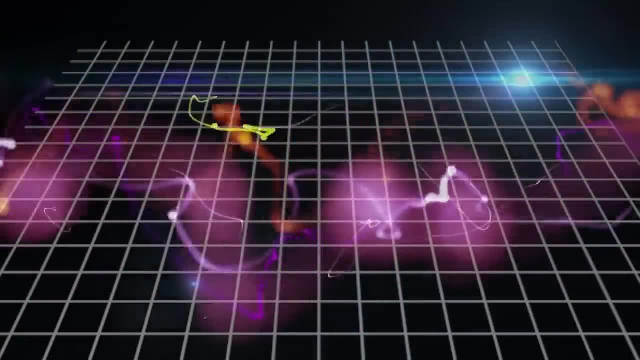 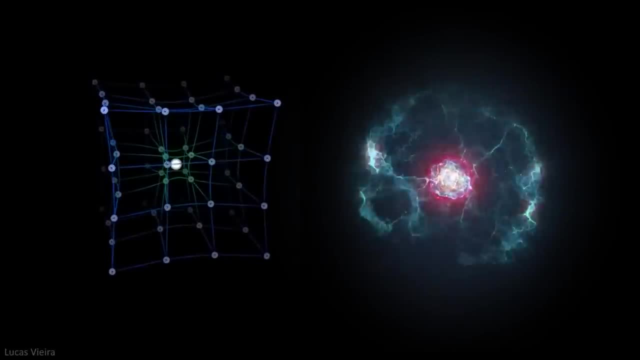 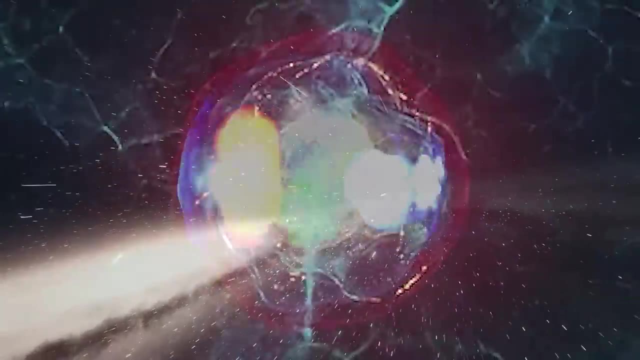 Additionally, Witton has noted that condensed matter physics is a rapidly growing field with many exciting open questions, and he's eager to contribute to this area of research. According to the Institute for Advanced Study, where Edward Witton is a professor on the emeritus, his current research interests include quantum duality, symmetries of field. 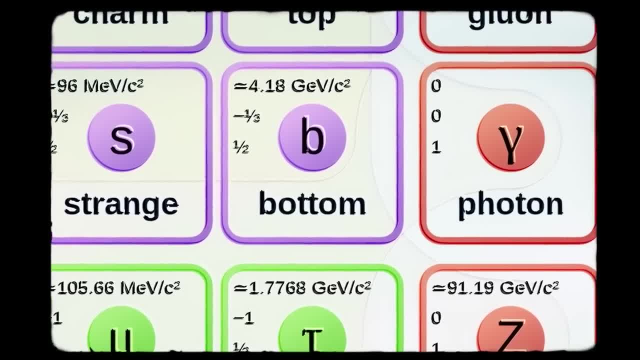 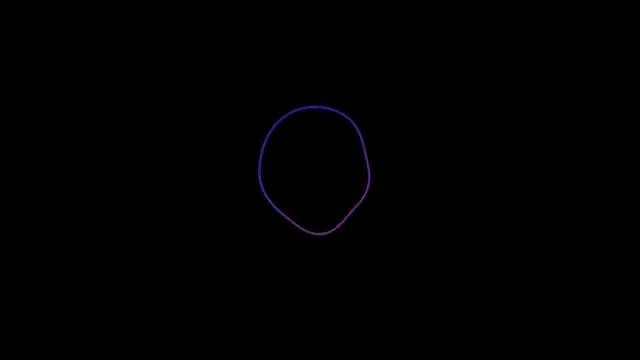 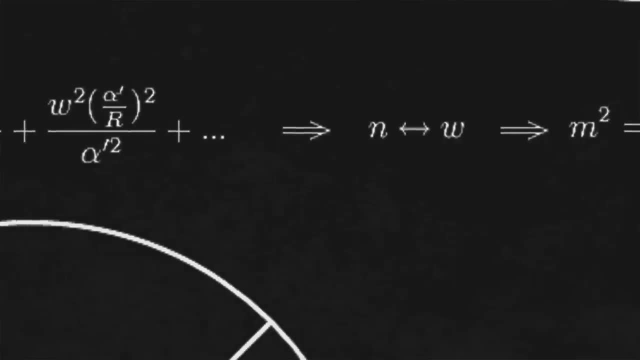 theories and string theories, which open new perspectives on particle physics, string theory and topology, an area closely related to the implications of string theory itself on our conception of spacetime. He's also exploring the relationship between quantum field theory and the differential topology of manifolds of two and three dimensions, as well as the connections between string. 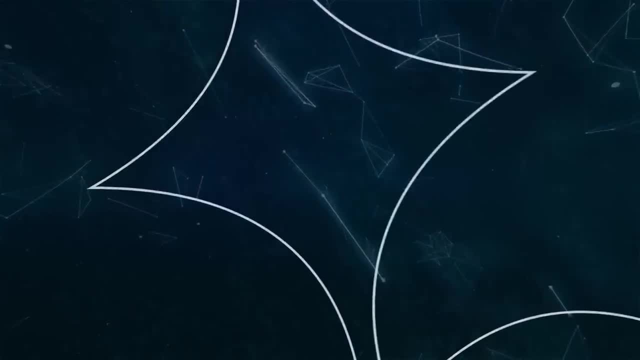 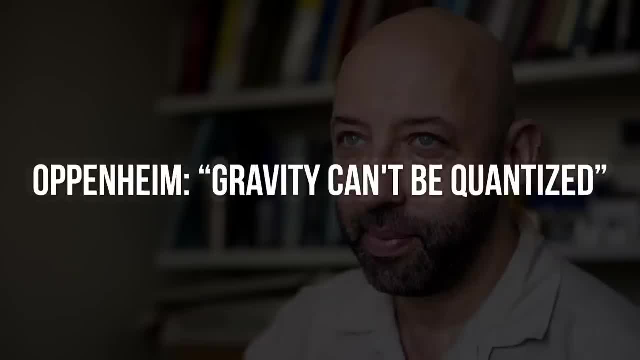 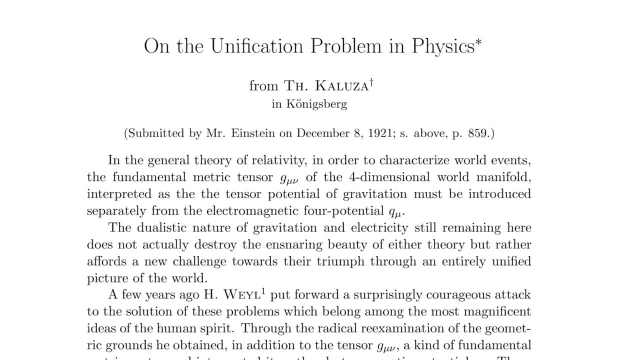 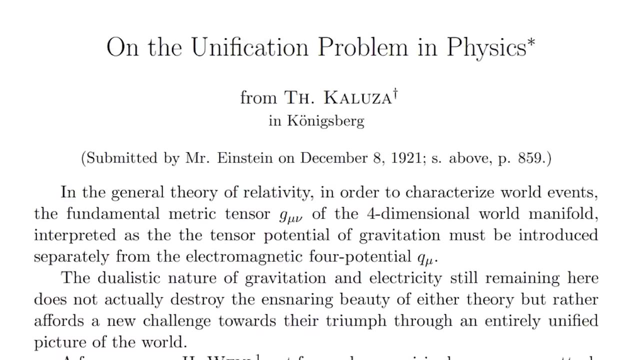 Oppenheim, Gravity Can't be Quantized. After decades of efforts and dedication of physicists and mathematicians such as Witton himself, science hasn't succeeded in its attempt to reach the unification of all theories. It's been unable to quantize gravity, which means, as we saw before sculpting an explanation. 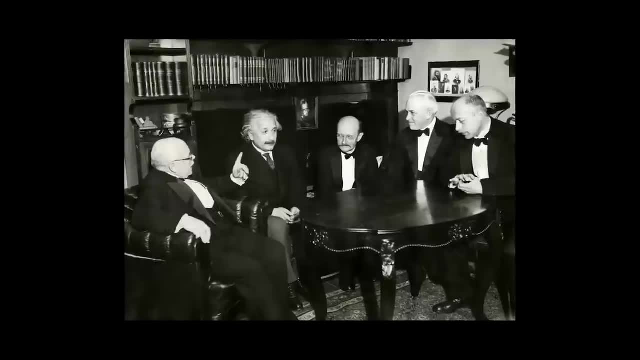 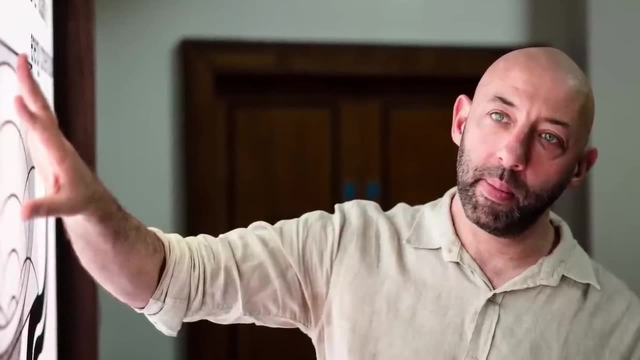 of gravity according to the rules of quantum mechanics, And there are already physicists who think it's not possible, like Jonathan Oppenheim, who is already working on a program at the University College London that explores post-quantum alternatives to the problem of gravity. 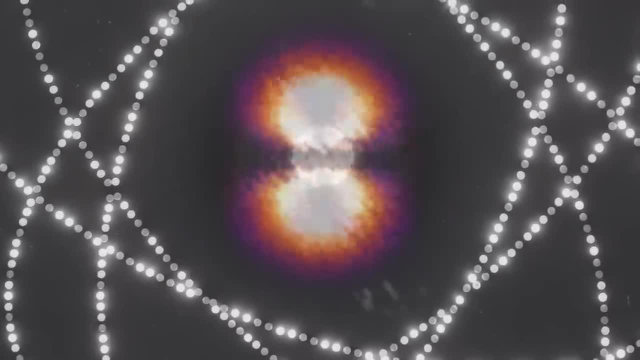 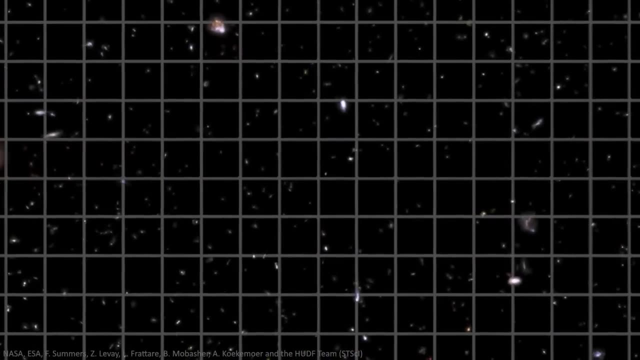 He works under the suspicion that gravity can't be understood simply by using the tools available in the quantum box. For him, even when the quantum view is ingrained, no one knows what the truth is. It's true that in the past century, physicists worked to gradually make sense of electromagnetism. 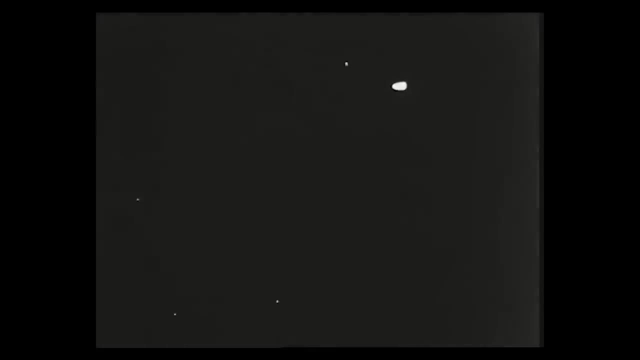 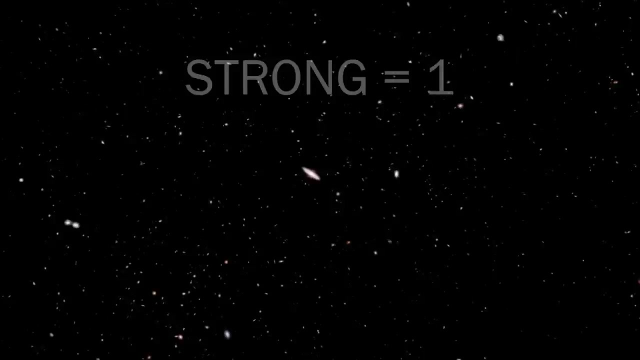 and the other two fundamental forces using the quantum framework, But the uncertainty expressed by Heisenberg's principle has made the quantum reality unsuitable when it comes to explaining gravity. Working with probability clouds instead of directly measurable magnitudes and irrevocable certainties has only led the equations toward unnatural infinities that end up being resolved. 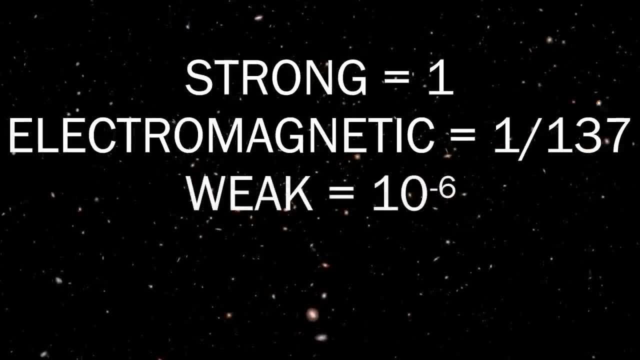 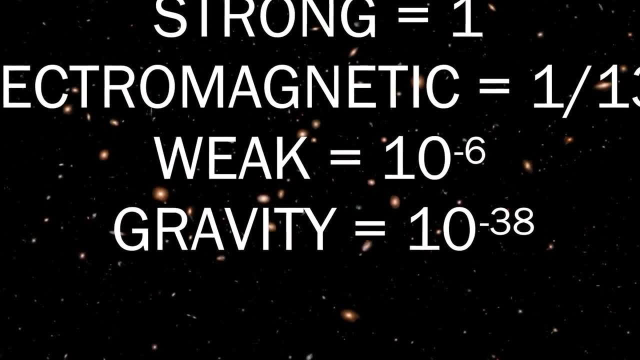 with less-than-elegant mathematical tricks. Witten's words about eventually redefining what space and time really are resound strongly here. When it comes to the three fundamental forces already quantized- they're not necessarily quantized- We are dealing with events that occur on top of the fabric of spacetime. 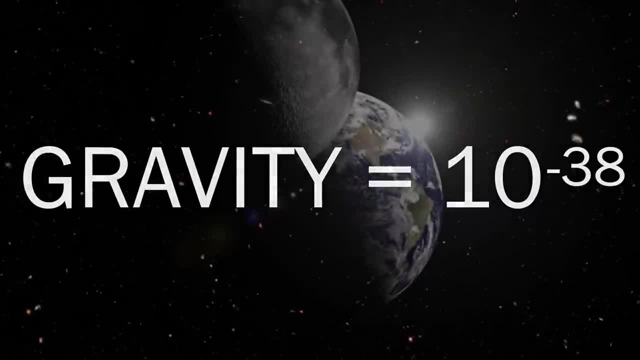 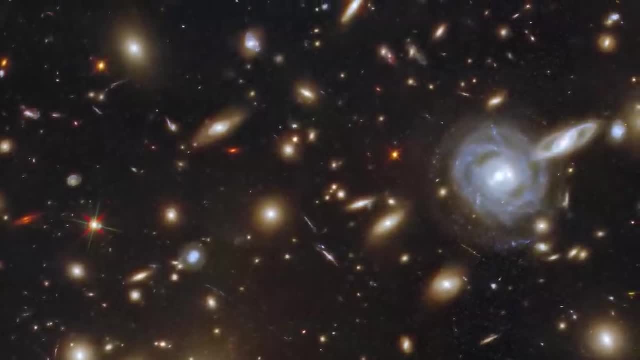 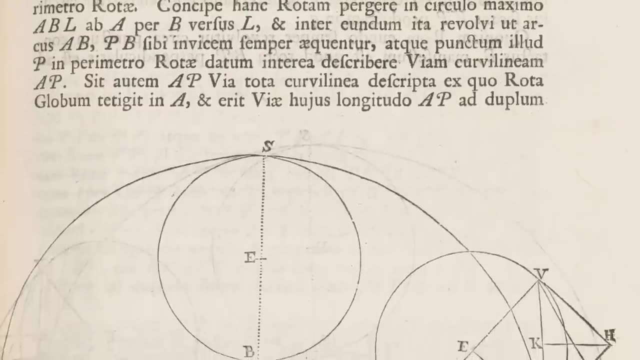 But gravity is a completely different story. It's a consequence of spacetime. If you quantize gravity, then you're effectively quantizing spacetime. This creates a bigger problem, since we would be developing quantum states on an uncertain foundation, as we leave behind the classical notion of spacetime. 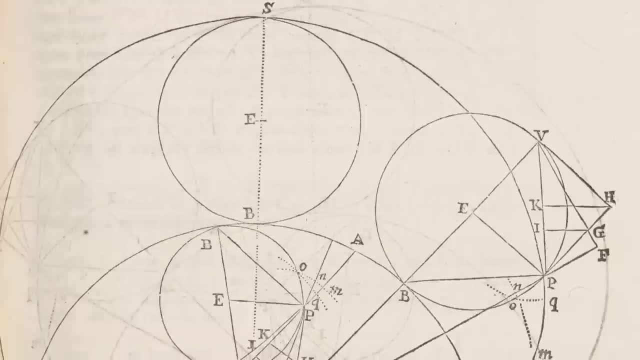 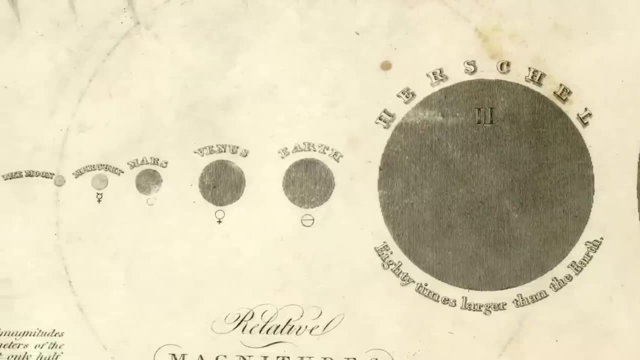 While Witten heads towards a deeper exploration of the topology and type of matter of spacetime, as proposed by string theory, A network of interconnected string loops, other physicists, like Oppenheim, uncomfortable with the mathematical acrobatics needed to make things work, opted for new ways of approaching. 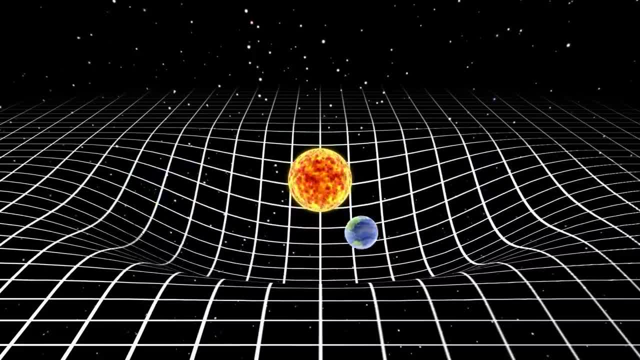 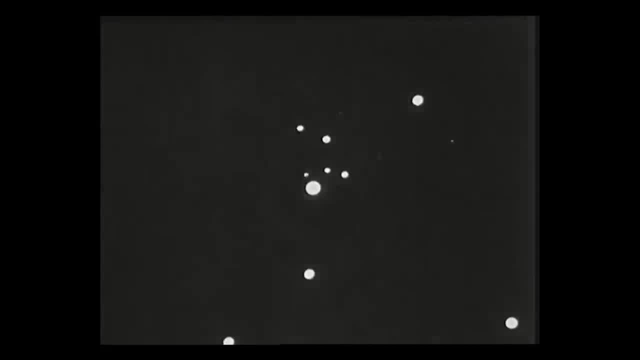 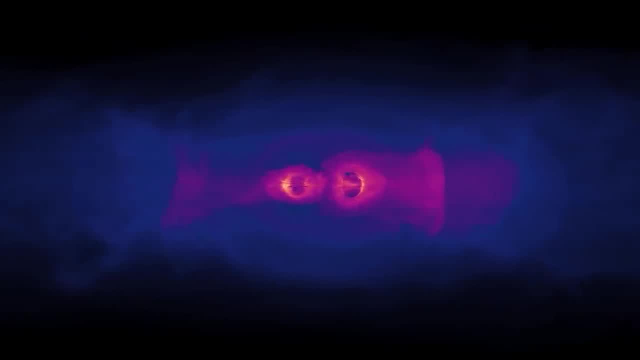 the problem. Oppenheim, originally a string theorist, grew less and less fond of putting all his eggs in the quantum basket. He even feels this has become dogma and scientists act like gravity should be quantized. Instead, he's been extending and exploring new alternatives based on hybridization. 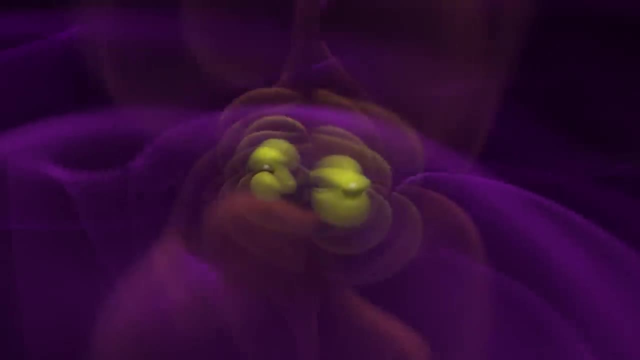 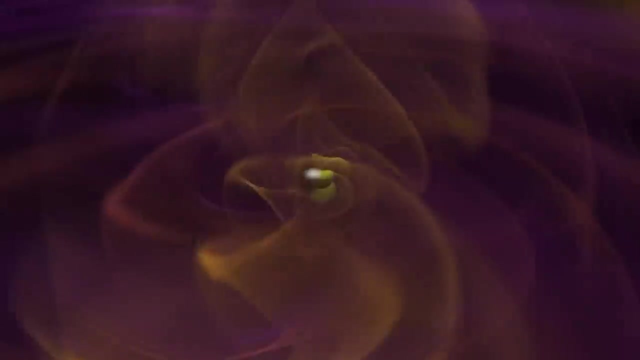 He doesn't fully bet either on the future. He's been trying to figure out what the future holds. He's focused on quantum or classical explanations as he tries to find a middle way that encompasses both worlds as foundations, basing his work on previous attempts on semi-classical dynamics. 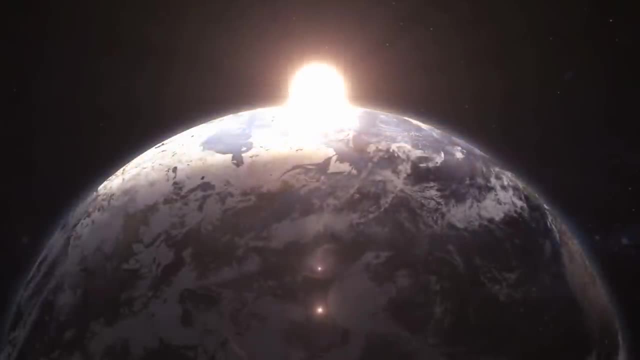 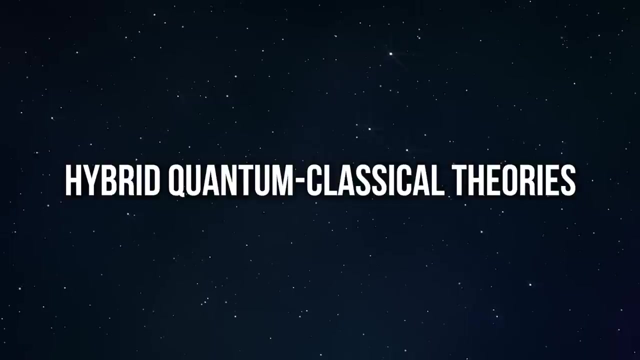 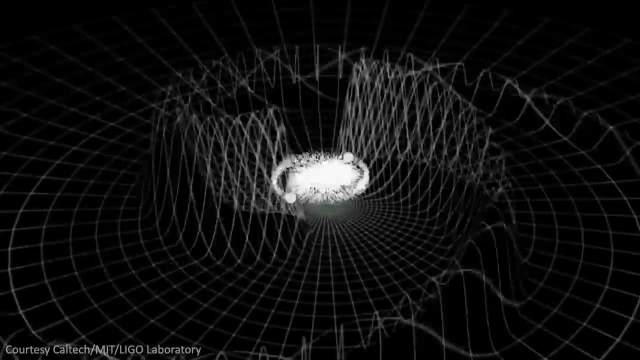 from the 1990s. According to his view, there shouldn't be anything about gravity that demands it to be quantized. So he tries to develop this new class of hybrid quantum classical theories in which gravity stays classical Oppenheim recognizes that gravity is indeed special, since it dictates the geometry and 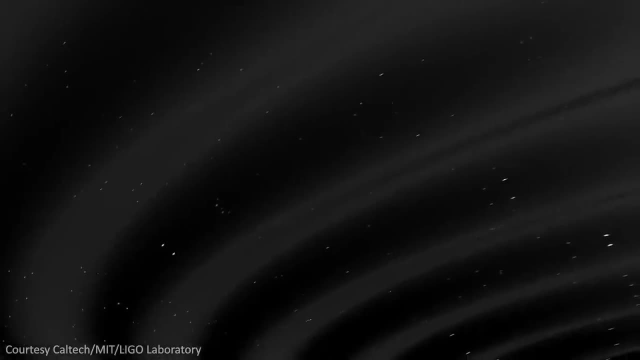 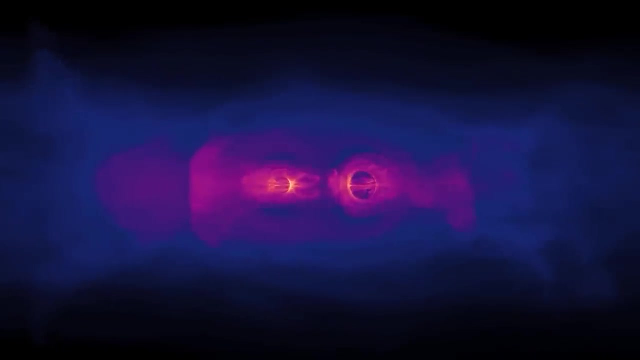 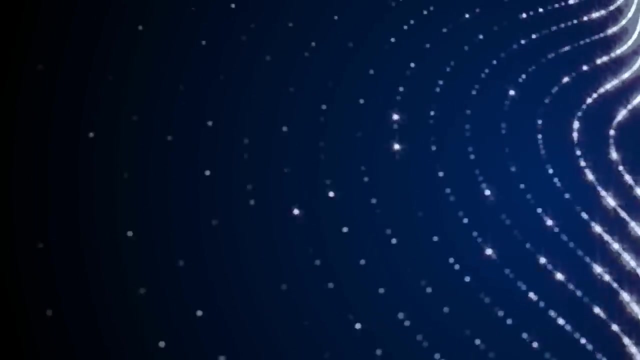 the curvature of spacetime itself, But this is precisely why he refuses to quantize it. Doing so makes us lose the background structure gravity creates. For Oppenheim, quantum systems and classical spacetime can interact in a consistent way. He and his students have constructed a hybrid theory that allows quantum particles to influence. 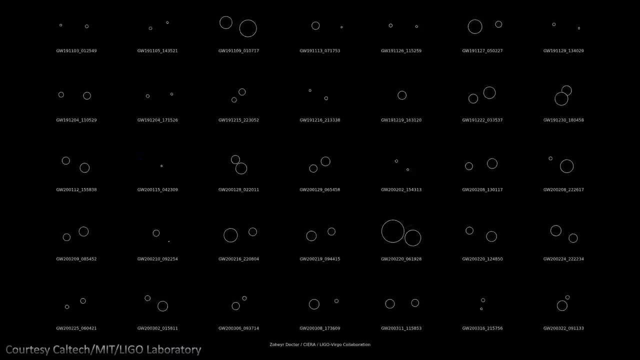 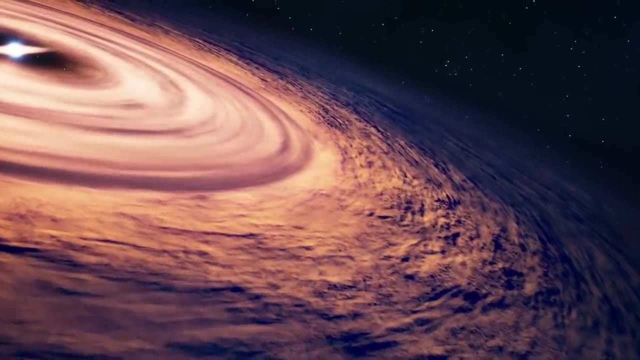 the shape of spacetime and vice versa, without violating the principles of quantum mechanics or general relativity. He based his departure from a quantum view of gravity on quantum mechanics. This is why he refuses to quantize it. However, the theory is based on a quantum view of gravity when studying the black hole. 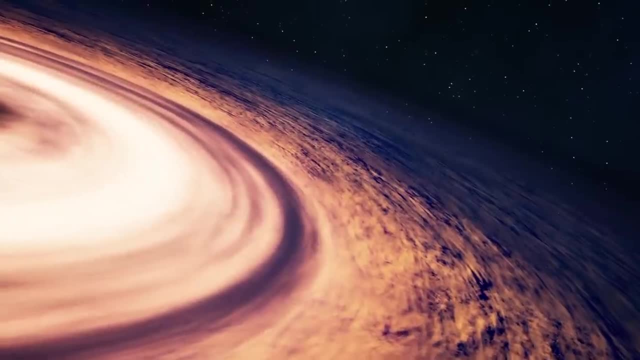 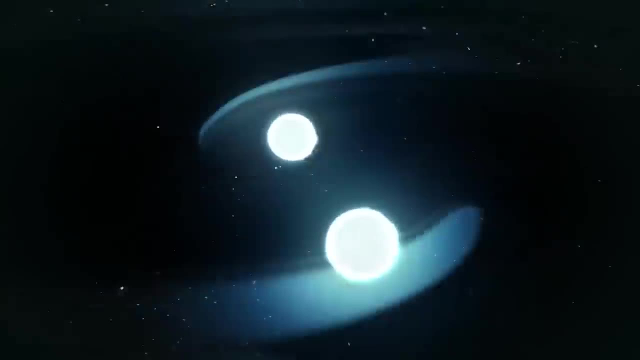 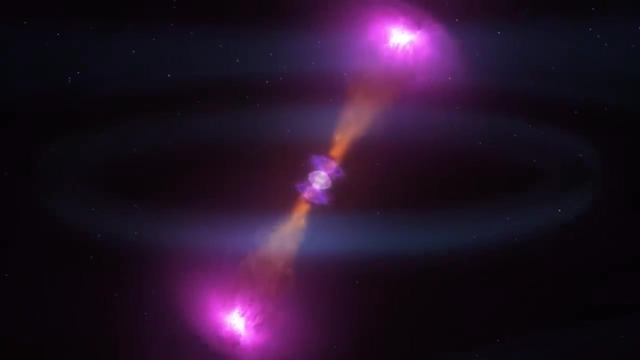 information paradox, a problem in theoretical physics that arises from the combination of quantum mechanics and general relativity. According to quantum mechanics, information is never lost. However, according to general relativity, information is lost when matter falls into a black hole. This paradox has been a source of much debate among physicists, and Oppenheim argues that. 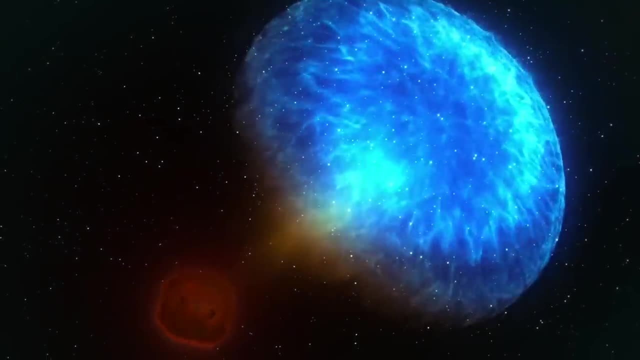 the only way to resolve it is to give up the idea that gravity is quantized. This is why he refuses to quantize it. However, according to quantum mechanics, information is never lost. This is why he refuses to quantize it. He argues that if gravity were quantized, then we would end up knowing too much, which? 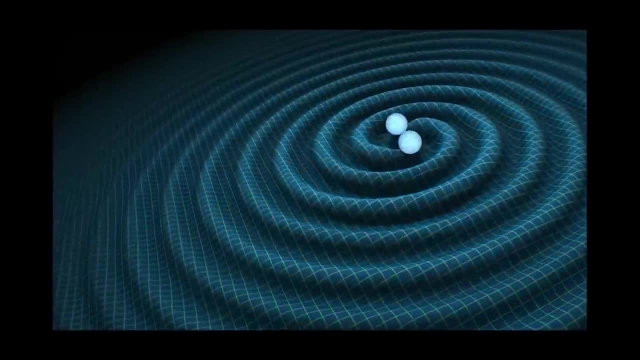 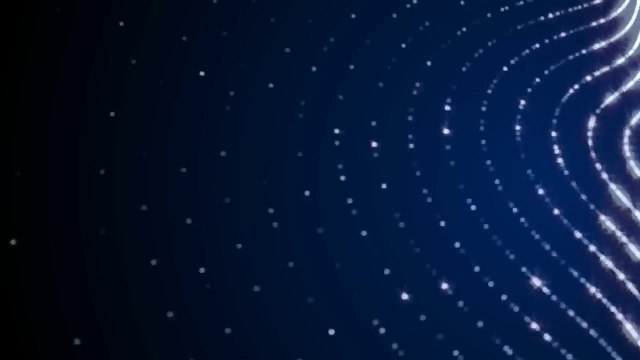 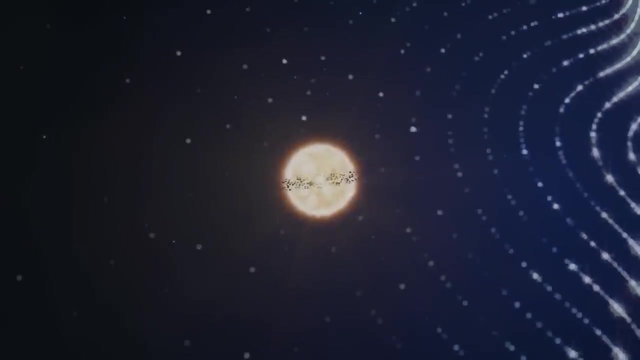 would break down widely accepted ideas from quantum mechanics like superposition. His proposal is a radical one, since it allows information to be lost in this scenario, and it's been met with skepticism from some physicists. To summarize his approach, Oppenheim is exploring the concept of a post-quantum theory of classical 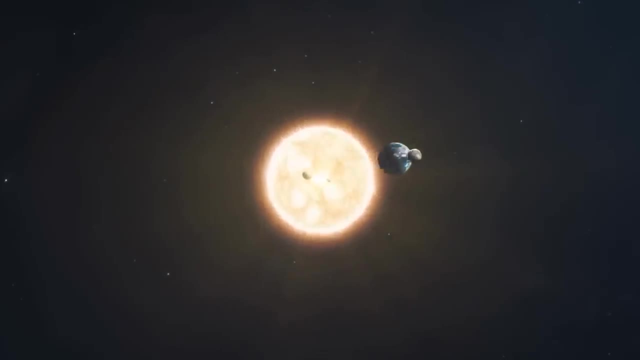 gravity. He proposes a novel classical gravity theory rooted in the concept of quantum mechanics. He proposes a novel classical gravity theory rooted in the concept of quantum mechanics. He proposes a novel classical gravity theory rooted in the concept of quantum mechanics. He proposes a novel classical gravity theory rooted in the concept of classical spacetime. 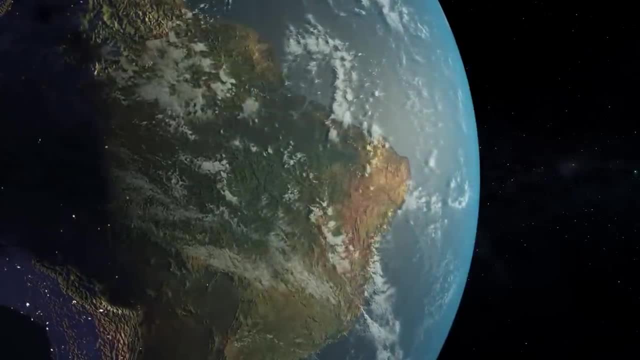 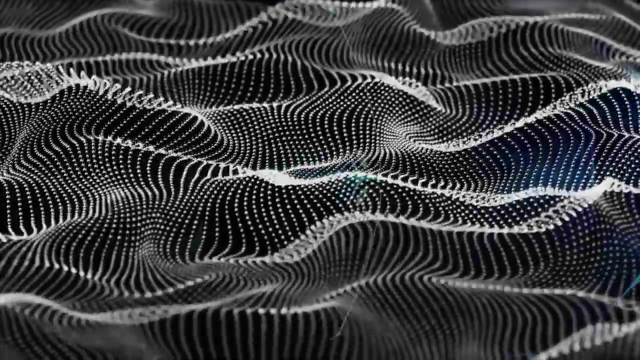 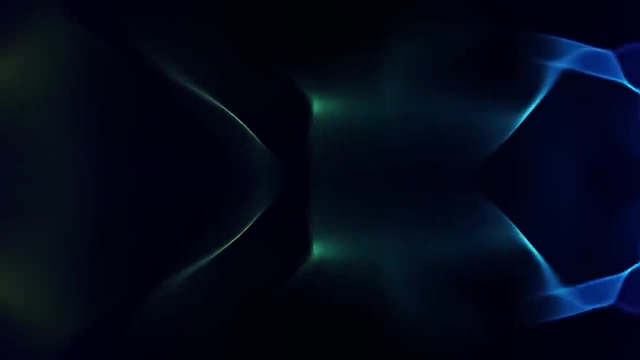 and the interaction of quantum systems with spacetime, leading to their classicalization. This theory entails intriguing consequences, including wavefunction collapse and information destruction. He suggests that his theory offers a solution to the black hole information paradox without compromising locality or energy conservation. 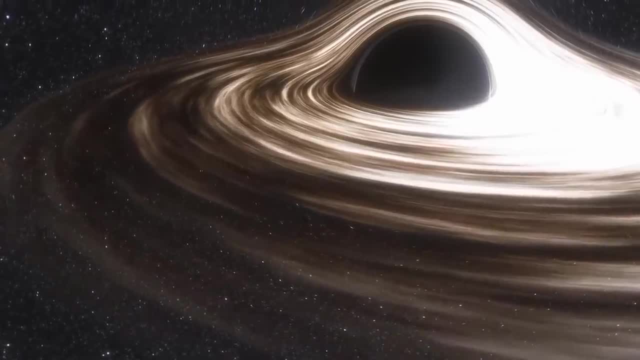 While Oppenheim's theory is still in its early stages and requires further development, it presents a thought-provoking approach to quantum gravity. He proposes a novel classical gravity theory rooted in the concept of quantum mechanics. He proposes a novel classical gravity theory rooted in the concept of quantum mechanics. 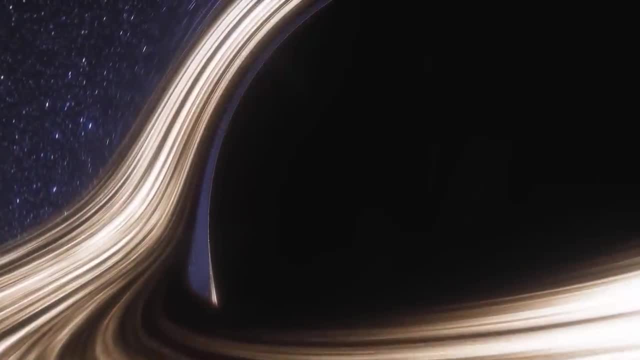 He suggests that his theory offers a solution to the black hole information paradox without compromising locality or energy conservation. This theory represents a writing technique that invites us to study reality in our own realization as we gather possibilities at the hands of a creative computer: tocho studies. 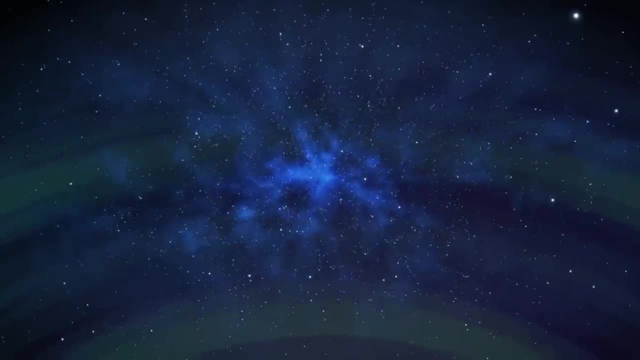 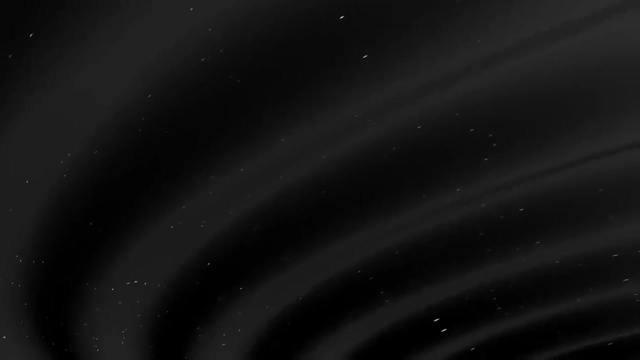 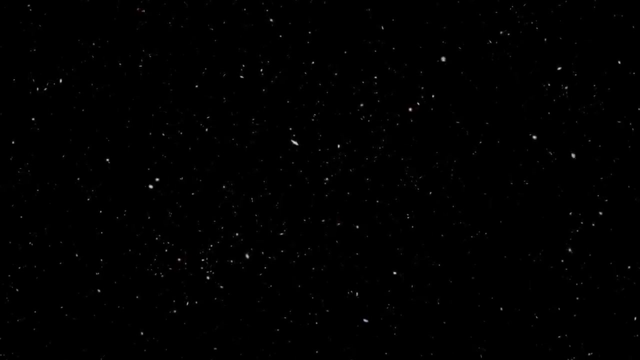 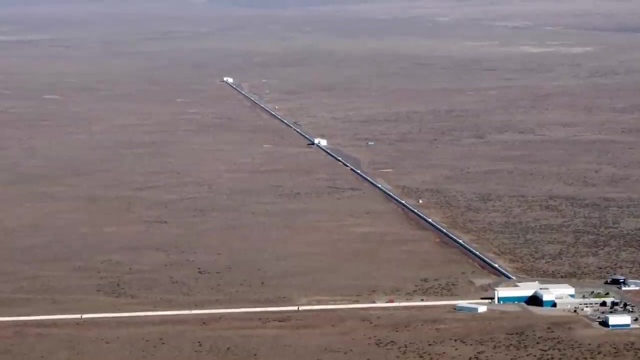 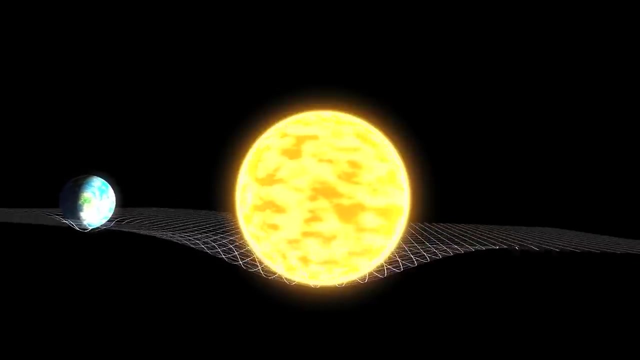 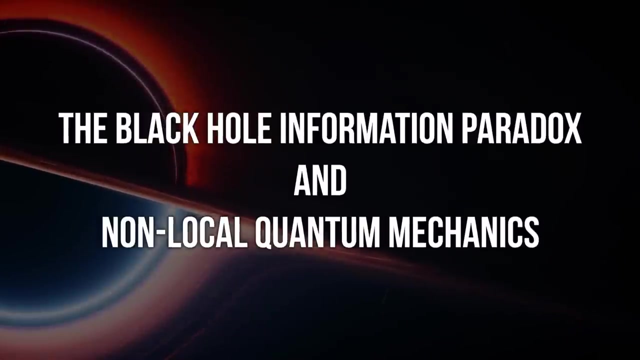 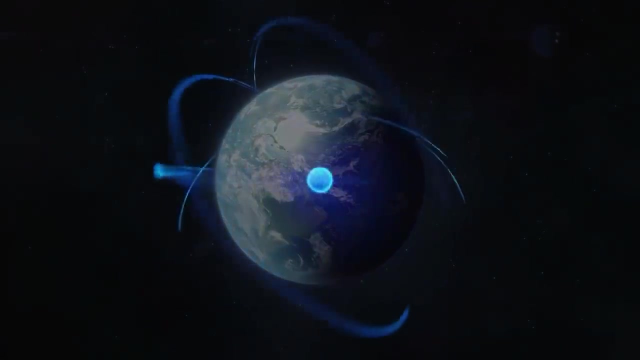 löwe illa, eliminate all these other sources of noise as much as possible. And, just like Witten Oppenheim believes that experiments on quantized gravity might be decades away, The Black Hole Information Paradox and Non-local Quantum Mechanics. Locality is a fundamental principle in physics that states that physical interactions cannot. 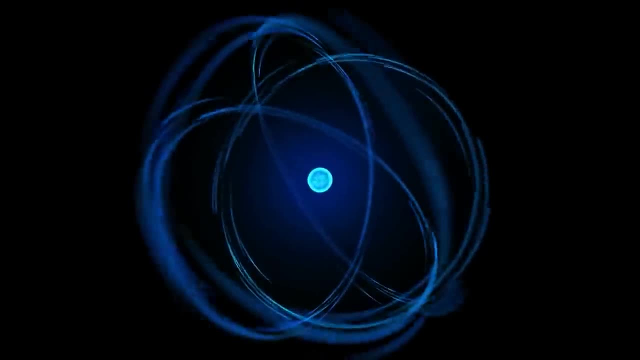 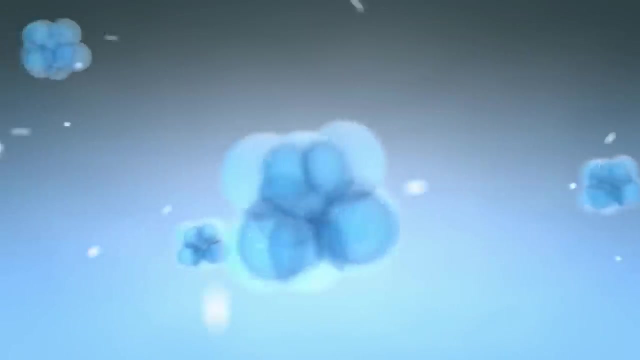 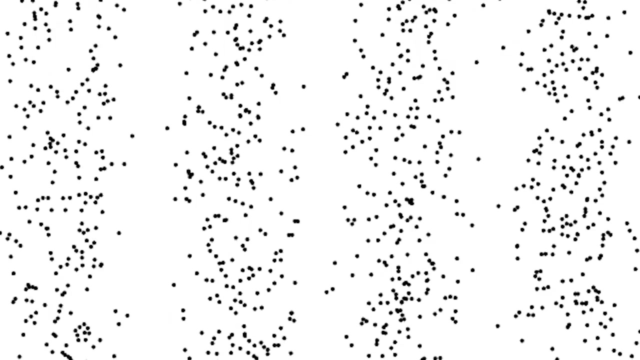 occur instantaneously over long distances. Objects down to the particle level can only interact with things that are next to them, either in direct physical contact or through a physical field that can transmit information between them. On the other hand, non-locality expresses the opposite scenario, one in which objects 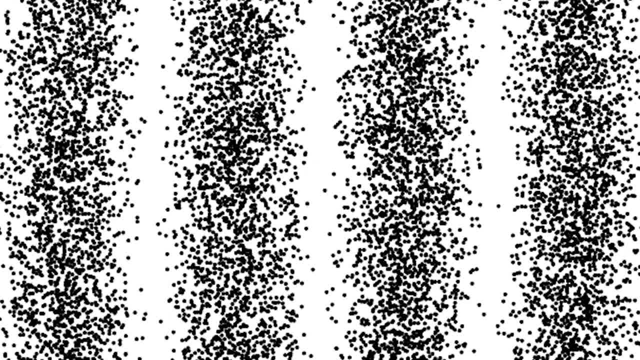 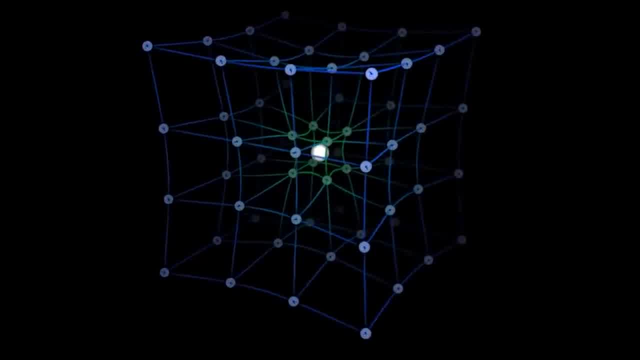 can interact with each other instantaneously, even if they're separated by a large distance. We have two types of non-locality. Physical non-locality is the idea that there's a real physical action that takes place between two objects, even if they're separated by a large distance. 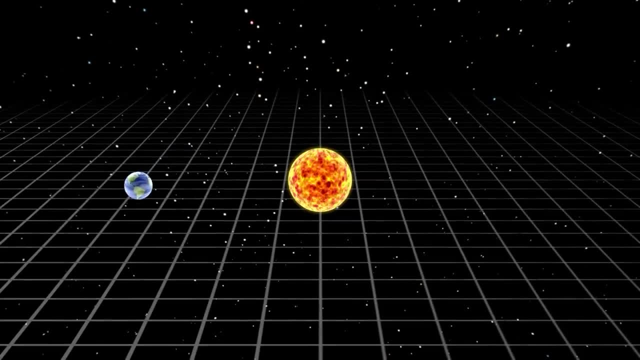 You may have heard about this before. In Einstein's theory, the idea of non-locality is that the non-locality is the idea that there's a design-spooky action at a distance. And then we have non-local correlation, which is the idea that two objects' information. 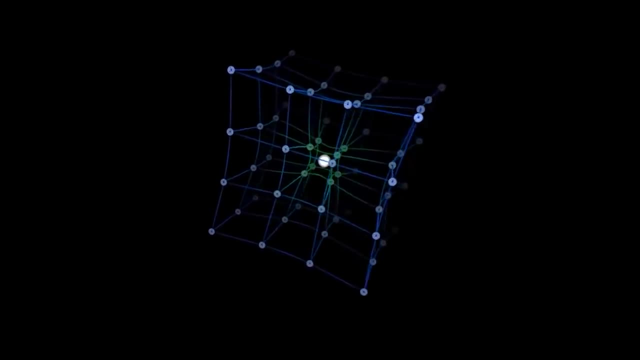 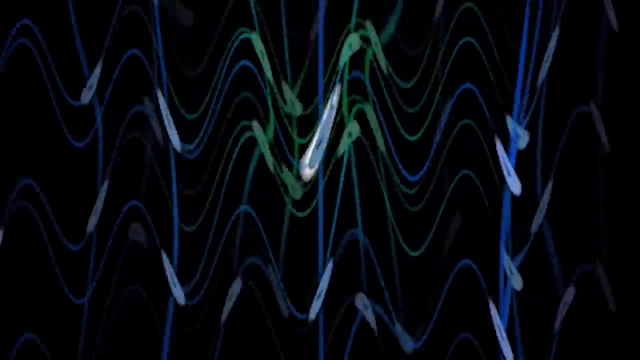 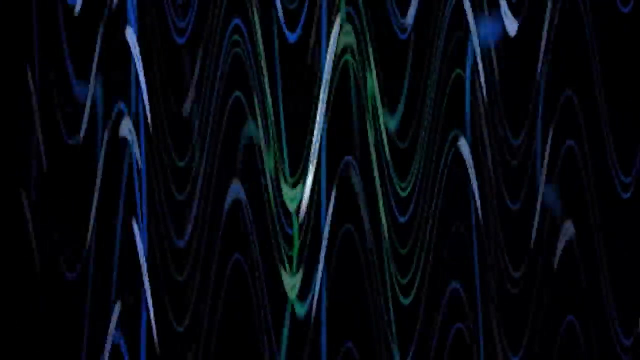 is correlated even when there's no physical action that takes place between them. In quantum mechanics, locality is particularly important because the wavefunction, which describes the probability distribution of a particle's properties, such as speed or position, can collapse instantaneously, regardless of the distance between the particle and the 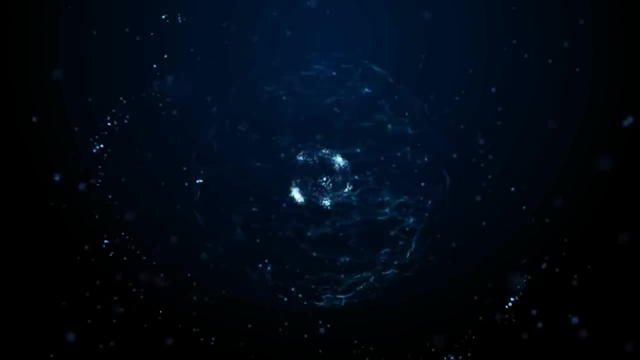 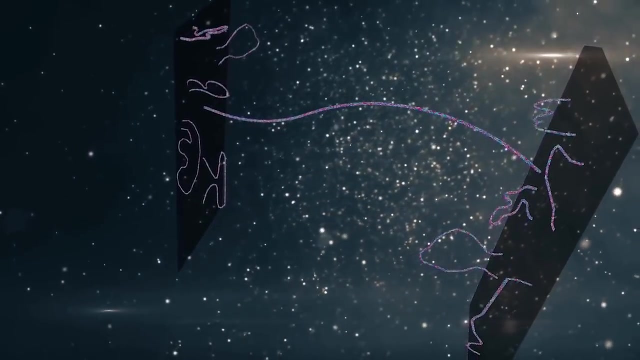 observer This instantaneous collapse of the wavefunction is the idea that two objects can interact with one another. The collapse of the wavefunction which occurs through and during measurement is what allows for quantum entanglement, where two or more particles become correlated in such a way. 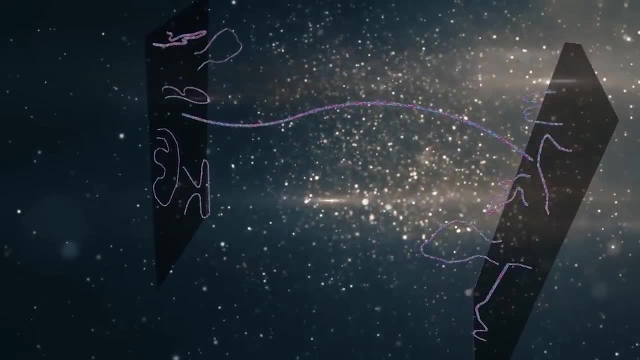 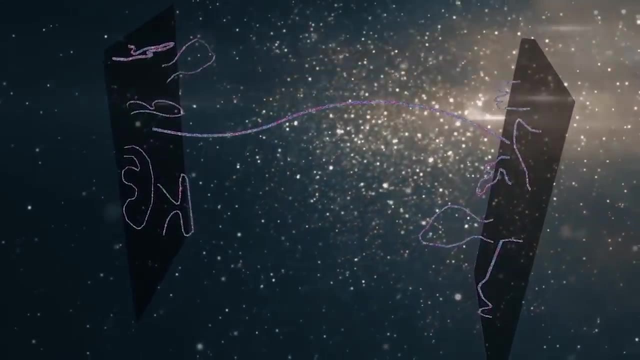 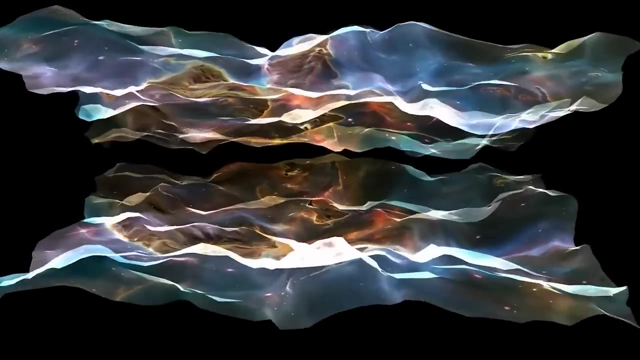 that they share the same fate, even if they're separated by vast distances. Oppenheim's proposed theory of quantum gravity does not compromise locality because it does not require the instantaneous collapse of the wavefunction. Instead, information destruction is a consequence of the extreme gravitational environment of 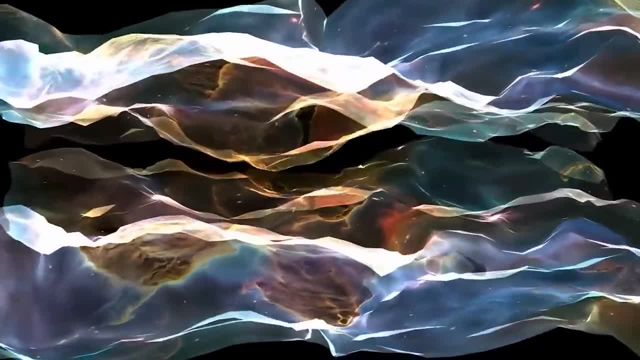 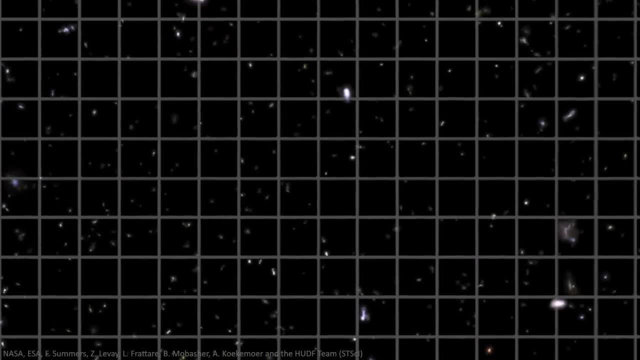 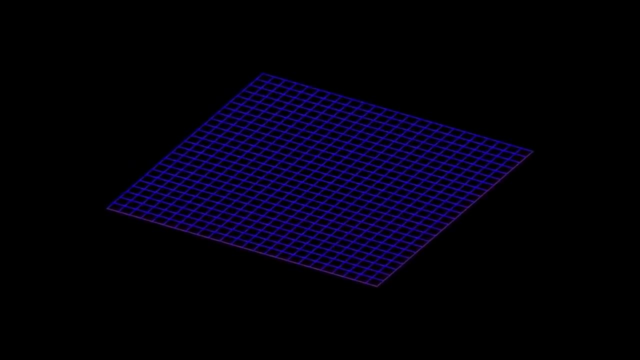 a black hole. In other words, information is not truly lost, but rather transformed into an inaccessible form. This happens because, as we saw earlier, Oppenheim's theory is based on the idea that spacetime is classical. A classical spacetime is not quantized and there's no need for a wavefunction collapse. 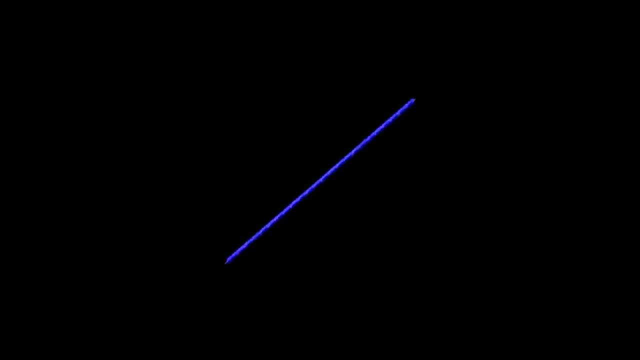 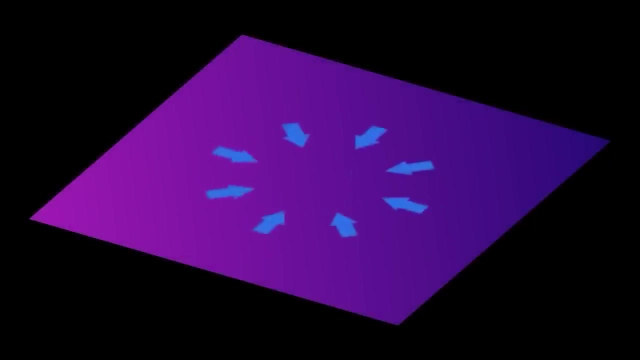 Instead of acting non-locally, information is transferred between quantum systems and classical spacetime through a process of decoherence. This decoherence is a natural, discrete-instantial process. This decoherence is a natural, discrete-instantial process. This decoherence is a natural, discrete-instantial process.